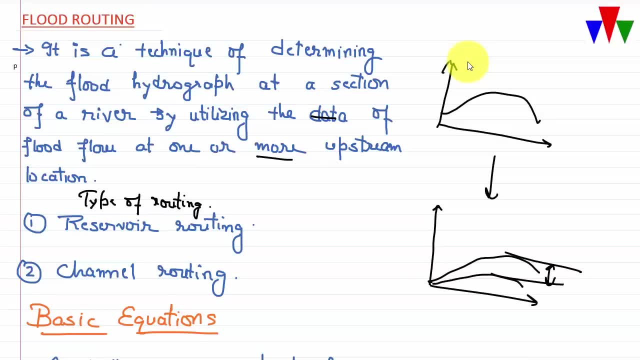 after it has passed through a channel or reservoir is called as flood routing. basically you route the flood or the incoming discharge. suppose what happens that in a river, this is your river end, here we have catchment area. all the water that is coming here, so in input hydrograph at this location will be- will have much higher peak discharge. 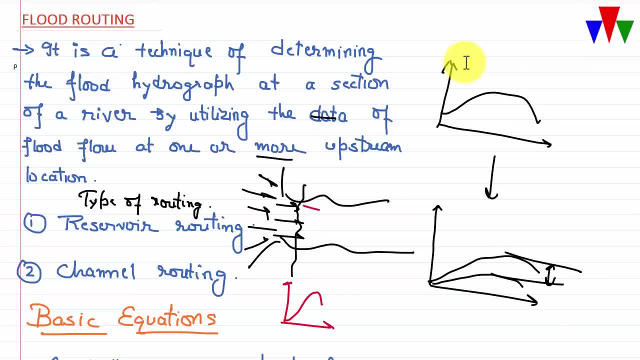 value what's. but what will happen? that as this water comes here, the storage will increase and the output discharge will be having a peak of lesser magnitude. so in a way we can say that if, If this is our input hydrograph at a point A here, then at point B, somewhere here, the output hydrograph will be like this: where we have this is your original hydrograph. 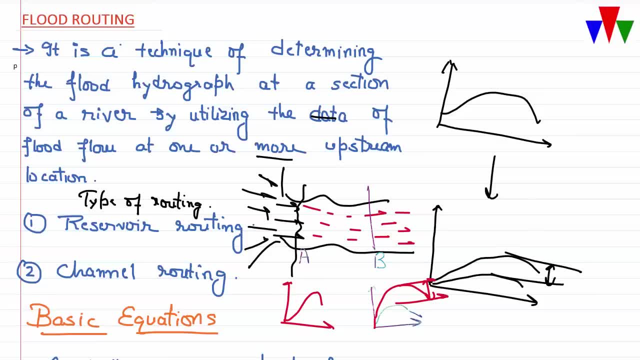 So this peak has been reduced. Basically, there are two methods of routing. One is reservoir routing and second is channel routing. Reservoir routing means that the water is stored in a reservoir and thereafter the discharge is allowed. In this way, the peak is reduced. and in channel routing, water is allowed to pass through a channel or river in which the storage increases and, as the flood receives, the temporary storage. 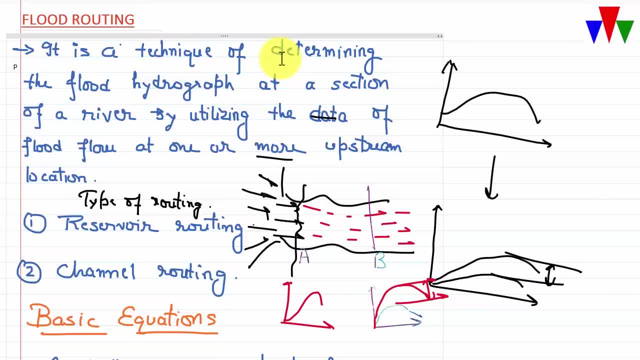 So this also leads to reduction in the peak discharge at the output section. Now flood routing is used in a lot of things. First of all, we can say that we can establish flood peak at downstream location, That is, we can predict flood and we can establish the effect of construction of reservoir on the flood, That is, how much peak of flood will be attenuated. 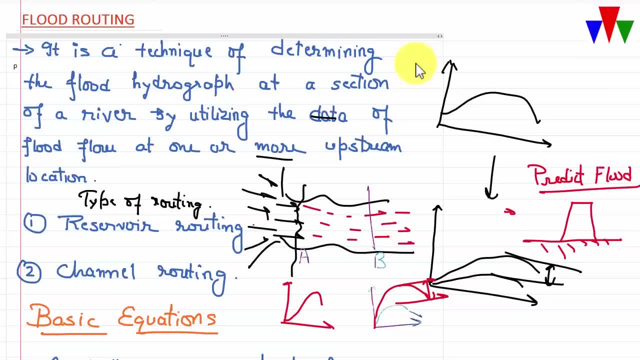 Suppose I make this dam, Then if water is stored in a reservoir, then we can predict the effect of construction of reservoir on the flood, That is, how much peak of flood will be attenuated. So if the flood is stored here and output is something here, then how much peak of discharge will this dam reduce can be determined with flood routing. 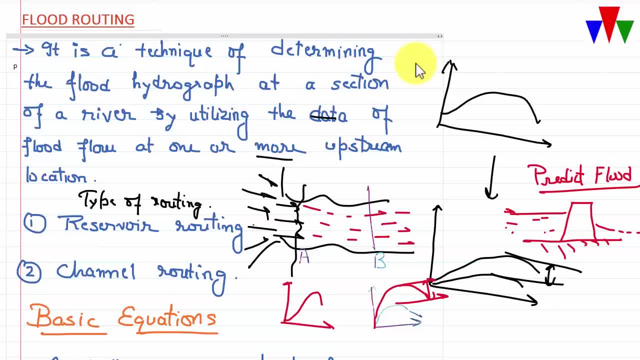 Here we can also determine the required height for flood protection. We can also predict the behaviour of the river after the change has been made in channel conditions because, as we are seeing, we also have a channel routing, So when the water passes through particular channel, It is said to be routed. 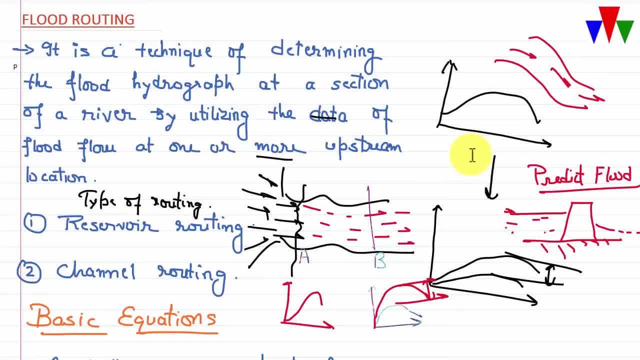 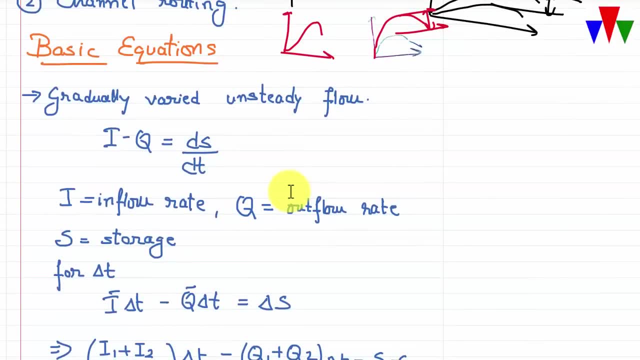 much peak will be attenuated. we will see it in further studies. so now let us see what are the basic equations which are used for flood routing. basic equation used is a continuity equation, which is input minus output is PS by DT. it means that change in storage with respect to time is equal. 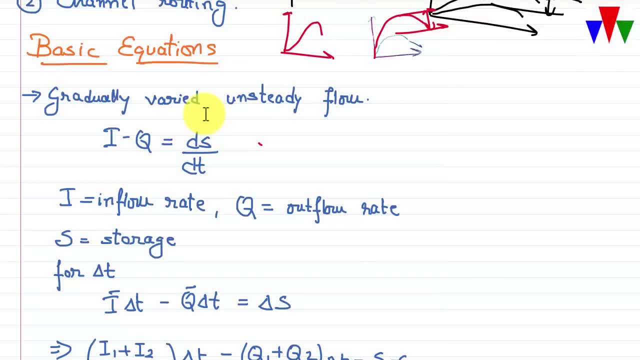 to input minus output. so this is your dam support reservoir. let me make- and here I have I and here we have Q and this is our s for storage. so input minus inflow minus outflow is equal to storage. now there are basically two techniques for using this routing. 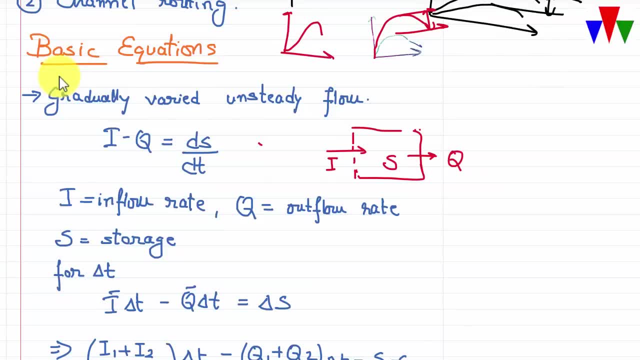 methods. first technique: I have not told you, that is a bit briefly, let me say this: lumped mass technique, lumped mass. in this technique we determine Q is equal to function of time, T at a given X location. and second technique is distributed routing, distributed. sorry, this is lump, not mass, this is lumped routing. lumped mass, you will study in. 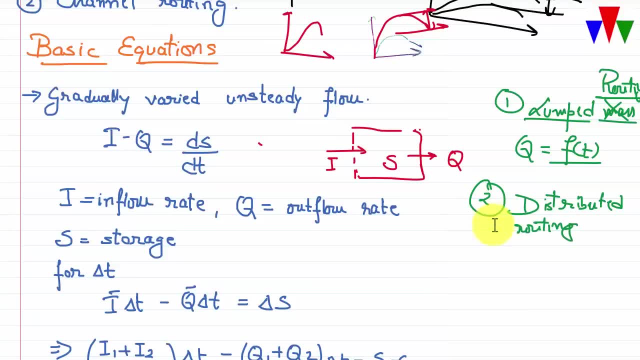 earthquake engineering. this is distributed routing. in distributed routing we find discharge as function of X and time T. the basic difference can be summarized as follows: in lumped routing, V is continuity equation. that is this equation. this is called lumped routing and distributed routing. we use the continuity equation with momentum equation, basically in: 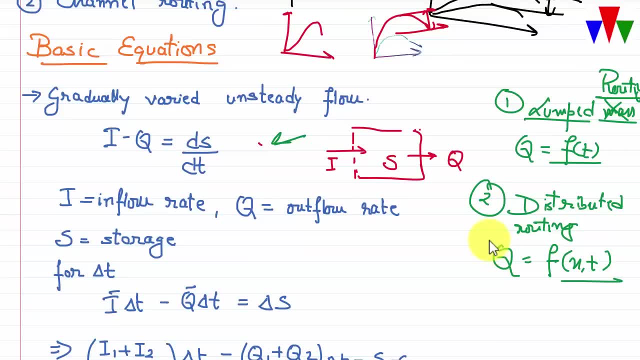 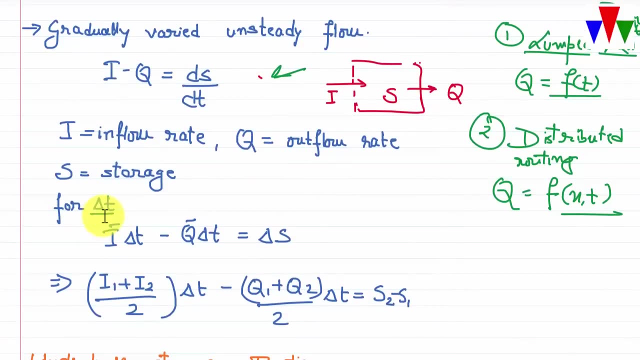 this chapter we will be studying about lumped routing only this distributed routing is not in our scope as of now. so let us see the original equation, original continuity equation that we were studying. let us say, for time T, I have input minus output is equal to 0.5. so this is the 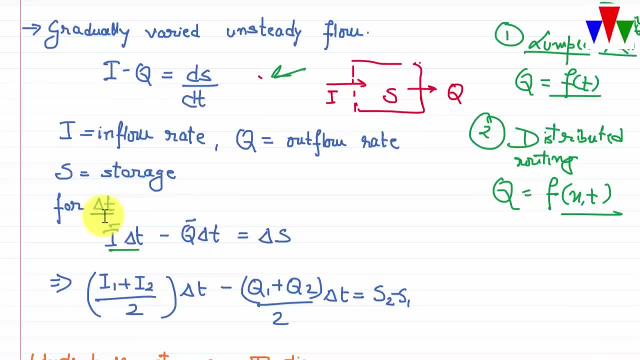 Singapore times a password for the boundary machine th. such is the use of B at 10: 0 and alpha plus below 0, because the point was 0. that значит this is more than 0. this version for B and the second combination is: eliminate any number and the nextАрен Order value in player is 0.07元. 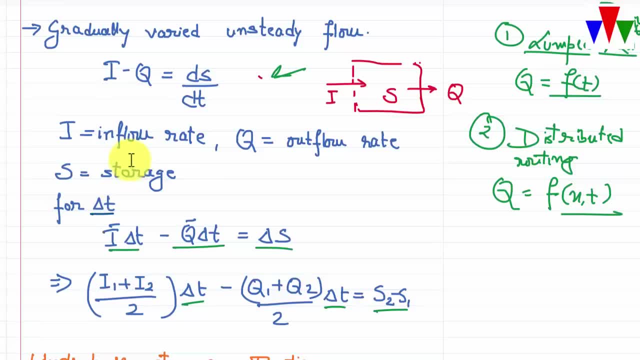 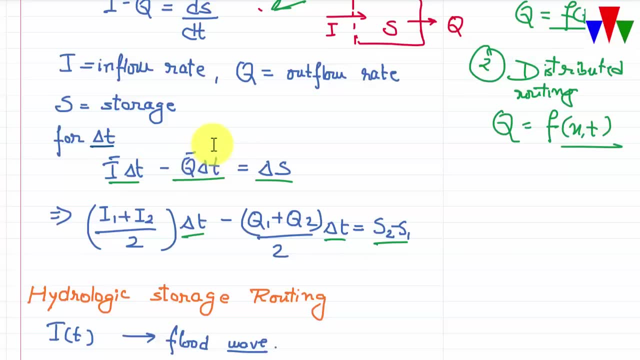 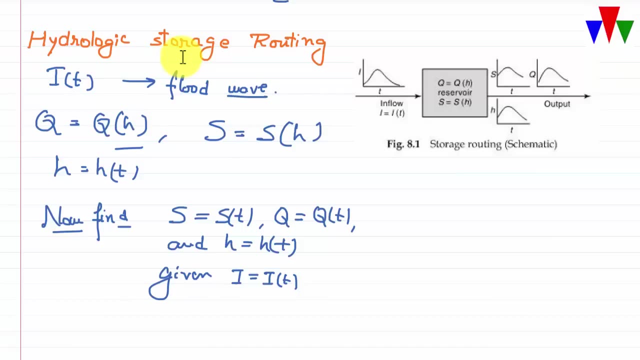 is equal to change in storage. so from this basic equation we will be driving all our routing equations. let us see how it is done. let us come to hydrologic storage routing. what happens? that in this routing method we are using a assumed level pool routing concept, that is, water level. 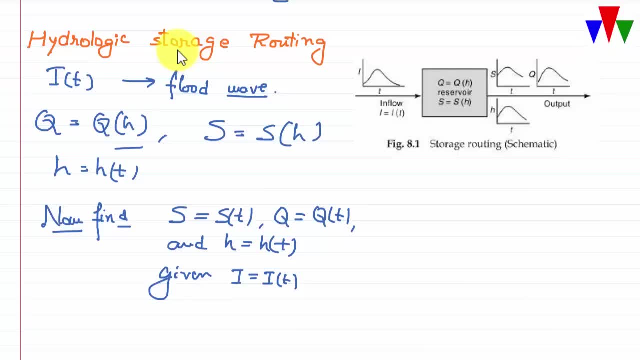 is assumed horizontal. in this case, storage will be a function of elevation only. it means that suppose you have a beer or spillway here like this and water level, water is stored behind this obstruction or whatever structure. it is now what happens that we can say in this case that storage in this, in storage in this type, 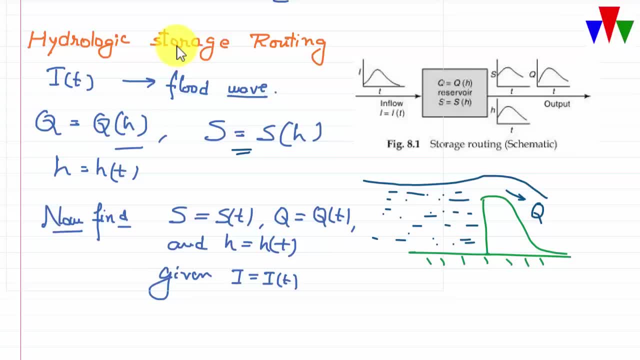 of structure is the function of height. so what is the level of water? through that we can determine how much water is stored. now we can also say that IT, that is, input, inflow of the wave- is a function of time T. in this diagram you can see that inflow of water is the 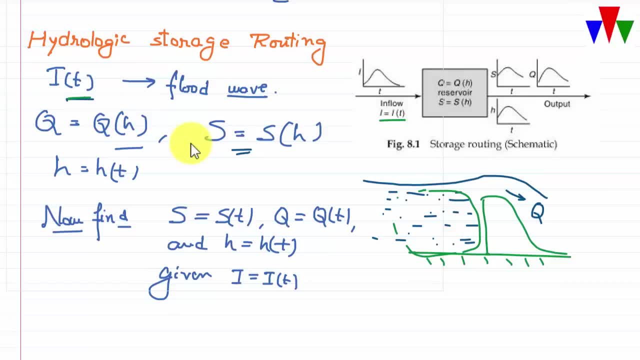 function of time T. and then we have our this reservoir here and after passing through this reservoir we get storage as a function of time T, discharge as a function of time T and height as a function of time T. so we have to determine these three things and the internal function of this reservoir is that we can determine storage as a function of. 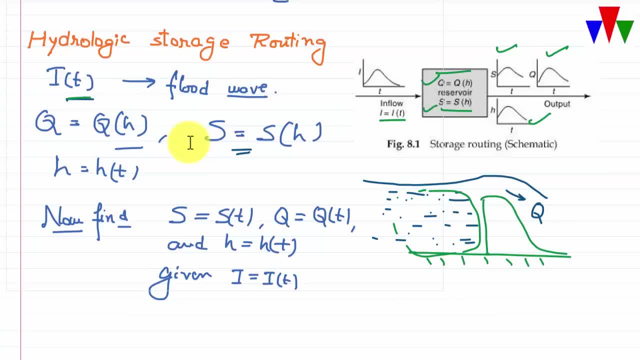 height H and discharge a function of height H. these two functions we know, and this inflow as a function of time T, we know. so from these three things, we have to determine these three things. this is a basic concept behind hydrologic storage, routing, that is, water is stored somewhere and when inflow. 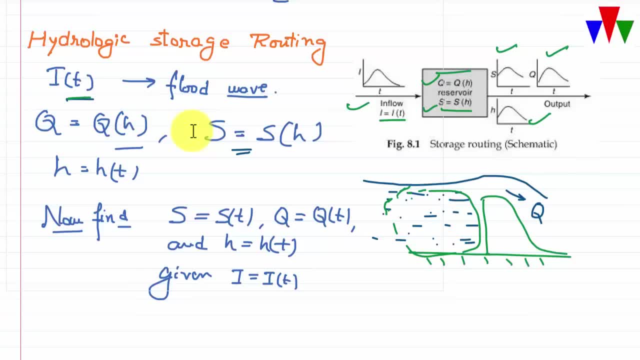 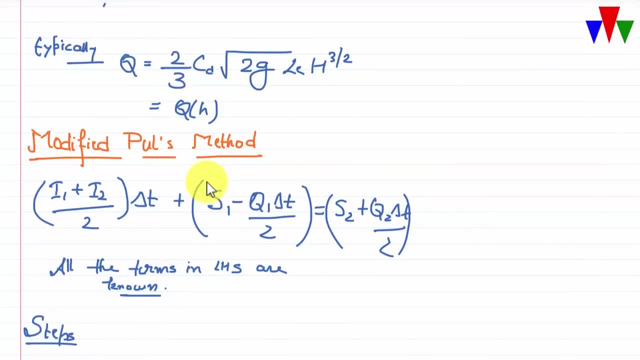 of water is there. the outflow function is to be determined in terms of time T. we can say that in our equation, in our structure, our discharge function for that reservoir was two by three, that is, I have written here: this is the discharge function, that is the. 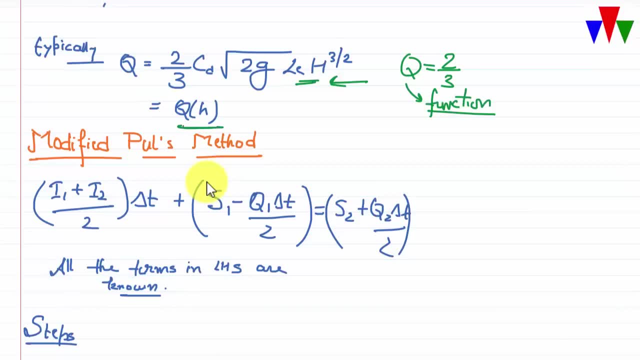 function of discharge with respect to your height, which we know that this is a function of Q of H. so in this case this equation is from fluid mechanics, where CD is coefficient of discharge, and how this has been derived you need to study there. through this discharge function and storage function of height H, we 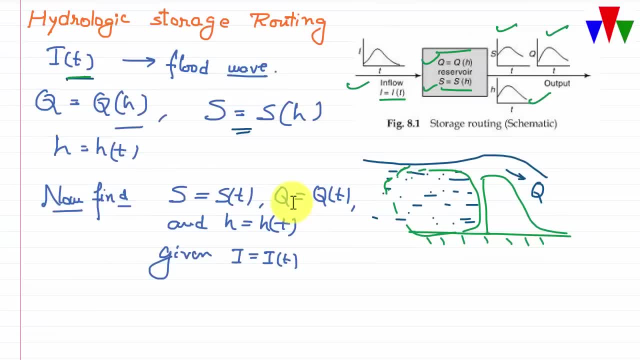 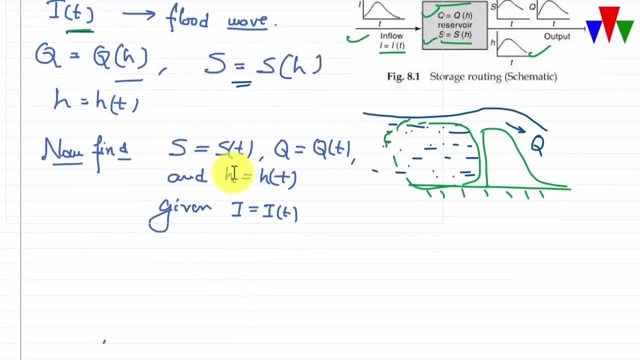 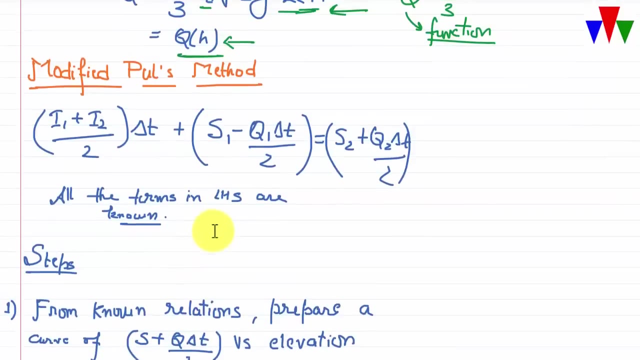 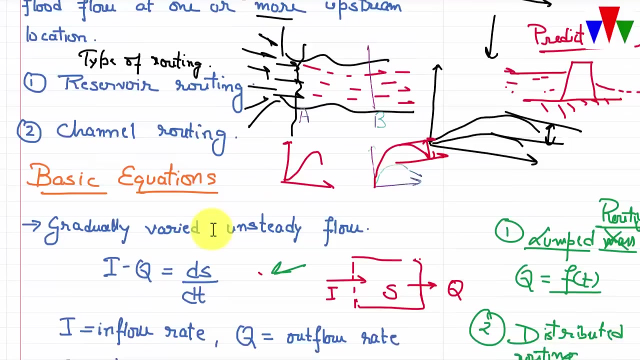 will be able to calculate inflow- we have here- and will be able to calculate outflow and height and out and storage of with respect to time T. now let us look at various methods of reservoir routing. reservoir is also comes under storage routing and this storage routing 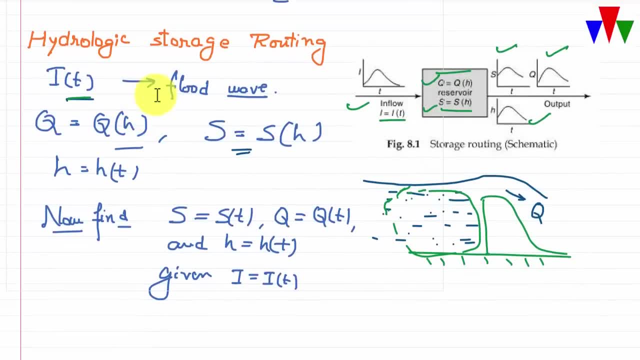 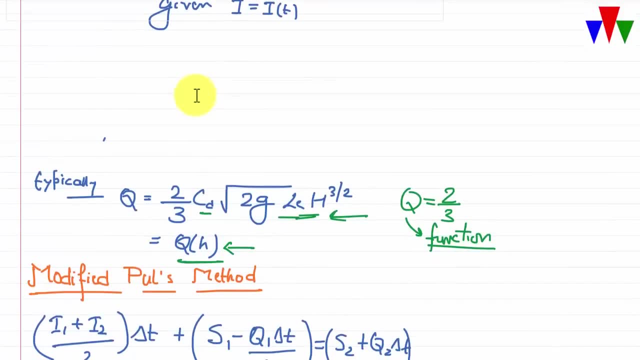 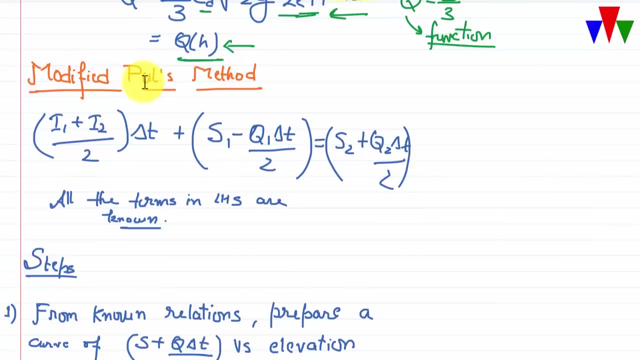 is basically one of the type of routing. so we have this thing. we have seen as a basic principle behind uh, how the routing is to be done, and now this is the method of routing. so first method we will be looking at is is modified. you can say it's full method in this case. 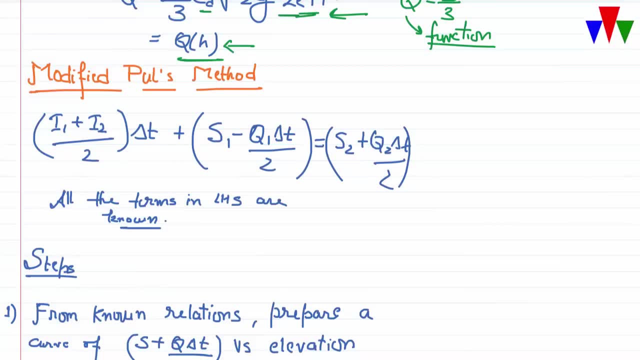 uh, basically this equation is modification of: uh, this equation let me write here. original equation is like this: I1 plus I2 by 2 Delta times inflow minus outflow. Q1 plus Q2 by 2 Delta T is a function of- is equal to change in storage, basically S2 minus S1. so rearranging these two things is going to be a very crucial step in using this method. 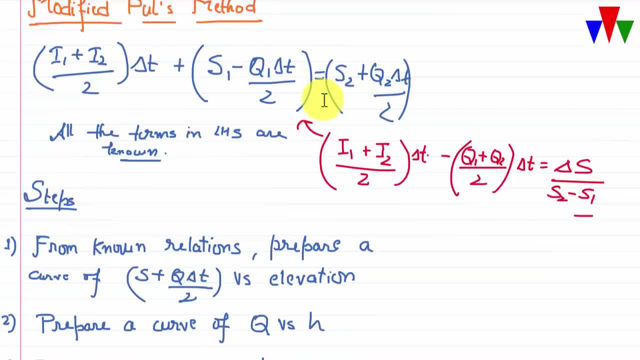 this we get. so what is the benefit of arranging the equation like this? we can, in this equation, we can say that we know this term, we know this term and the only unknown that we don't know is here. we know q1, s1 and delta T, so we have to. 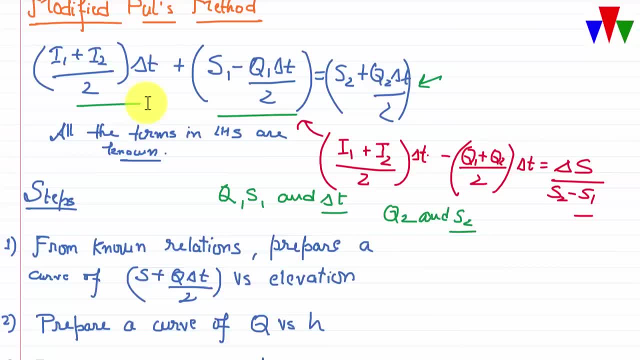 determine q2 and s2 after time T. there is discharge function and storage function after particular interval of time T. so we have rearranged this equation in this way. now the given thing. let us write once again: we know Q as a function of H, discharge as a function of H. we know storage as a function of H. 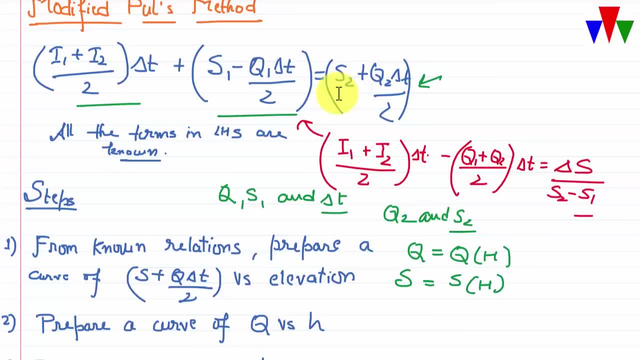 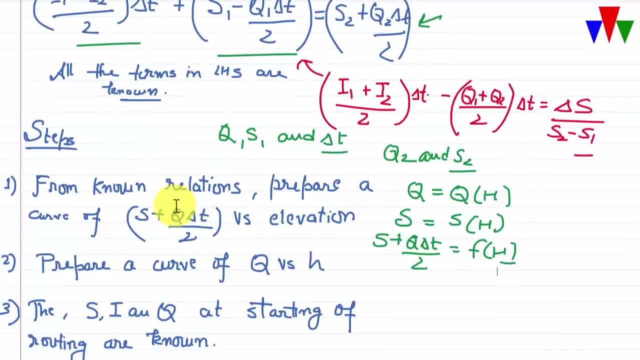 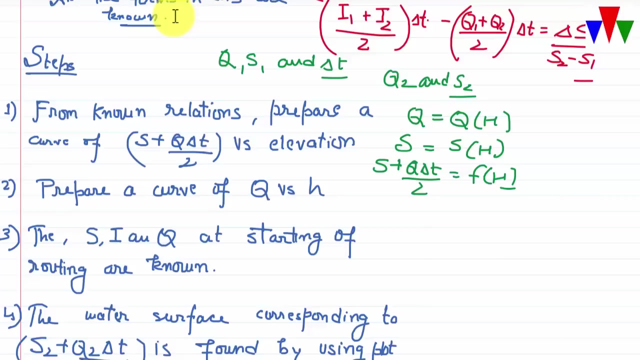 because it is reservoir pool or storage pool loading. so basically, s plus Q, Delta T by 2 is also known as function of H. by combining these two things now there are, let us study. what are the steps from, what are the steps to determine this? the various 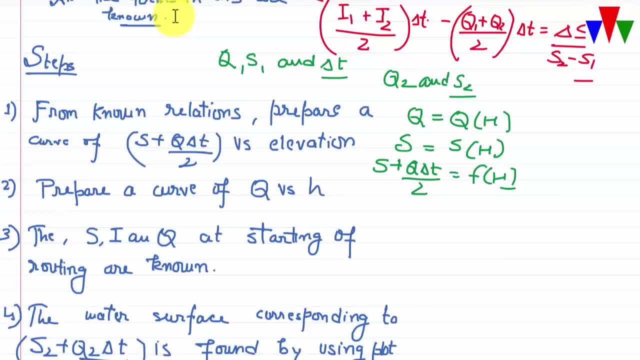 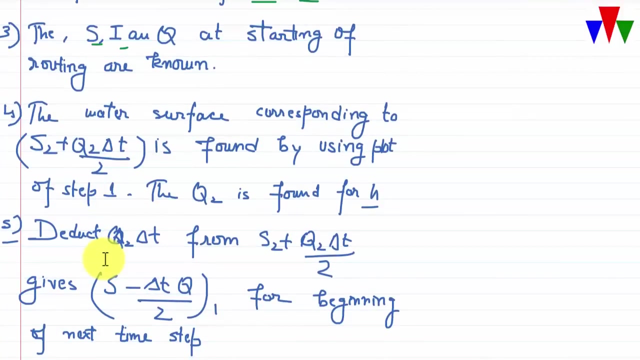 steps in loading. for the first time, interval, delta T, we can say that from the known relations we can prepare a curve of s plus Q, T, Delta T by 2 versus elevation. that is this thing. now we also have curve of Q versus H. so storage, inflow and 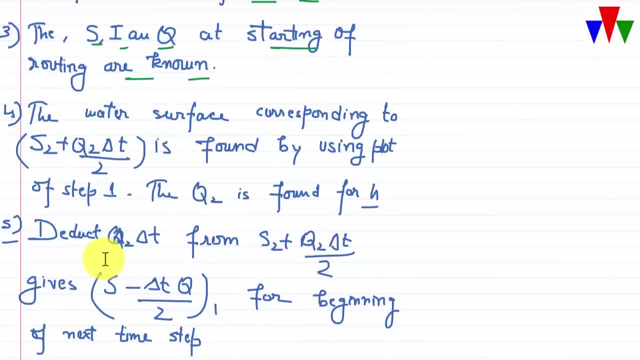 outflow at the starting of routing are known. this is a clear fact. the water surface corresponding to s 2 plus Q 2, Delta T by 2, is found by using plot of step 1. Q 2 is found for. so what you can do, we know we can find H for this. 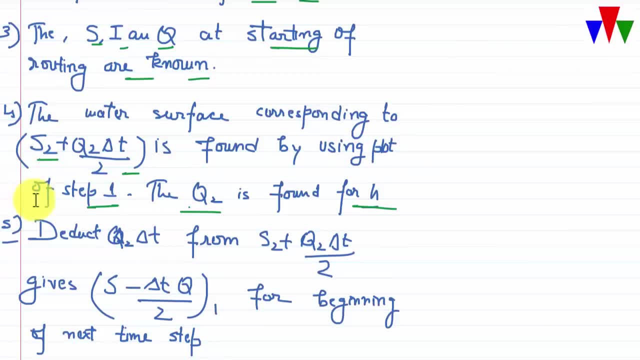 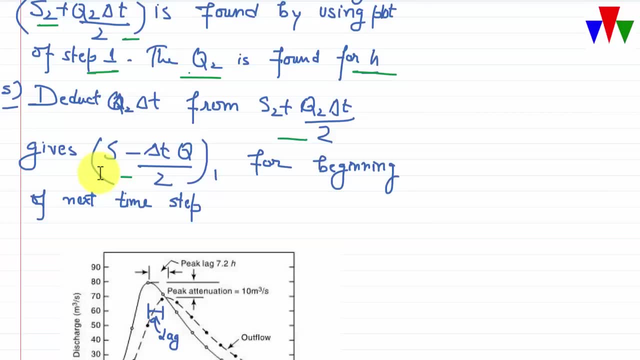 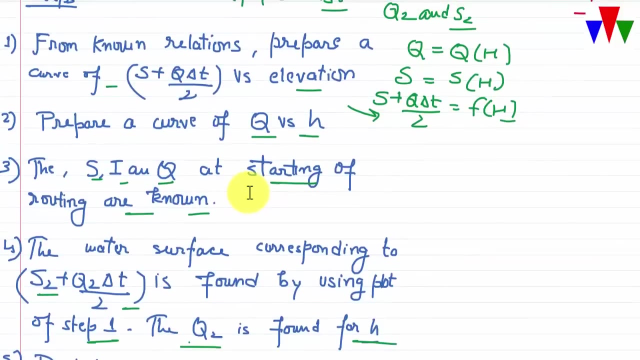 function from H we can determine Q 2. so now we can deduct Q 2 Delta T from this to get this for the beginning of next time. but we have seen. let us go through it once again: I 1 plus I 2 by 2 Delta T and s 1 minus Q 1 Delta T by 2 delta T is 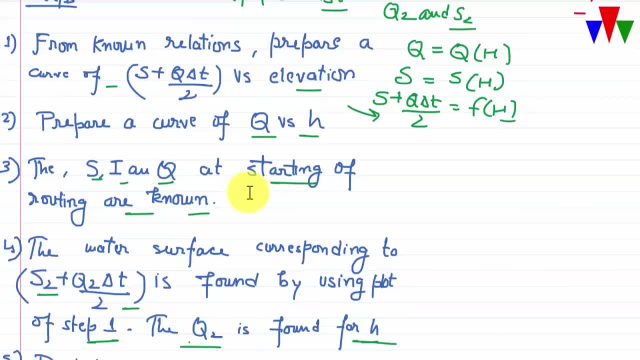 known what it is saying, that at the starting of your curve, at the beginning, you have I 1 plus I 2 by 2 Delta T. you know this term, okay, and all you also know s 1 minus Q 1, Delta T by 2. so you can determine s 2 plus Q 2, Delta T by 2. you can. 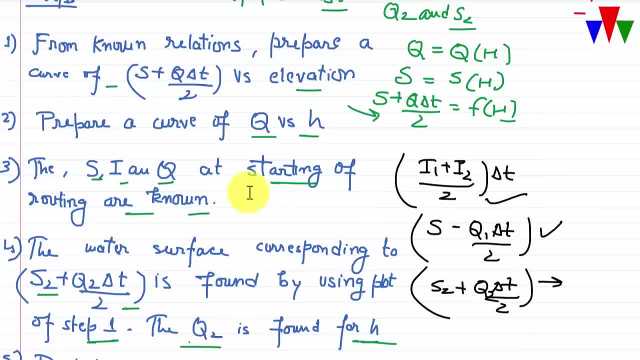 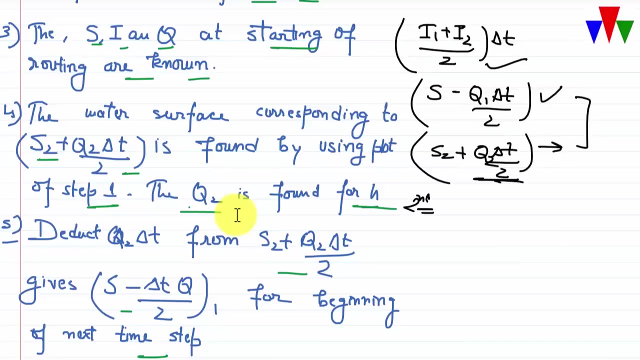 determine this from the relationship of this s Q Delta T by 2, we can determine H. this is this, this we have to determine H corresponding to this, that is, discharge elevation relationship. so for the next increment, this is a step 1 for the second step, other for second increment. basically, what we can to do is that we 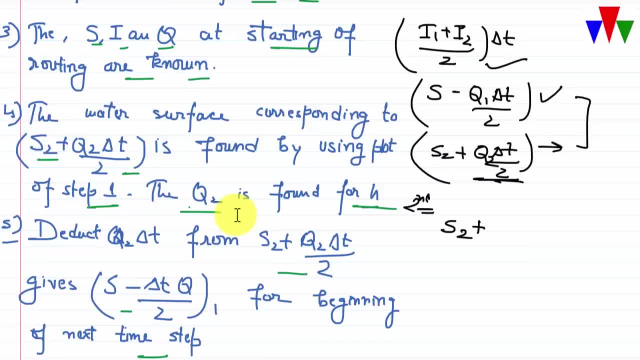 can subtract. we already know the value of this one. so we can subtract s 2 Q 2 Delta T by 2. this is original minus Q 2 Delta T. we can subtract this to get step 4, next step. basically, let me just briefly tell. 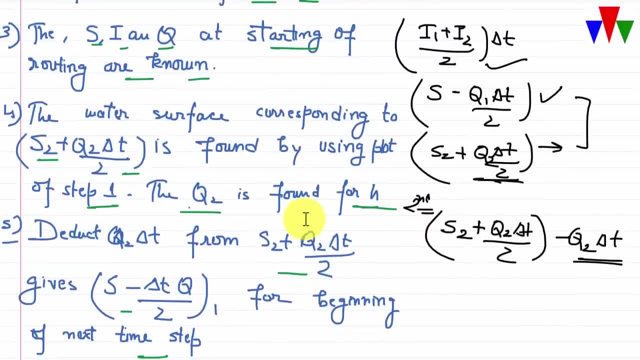 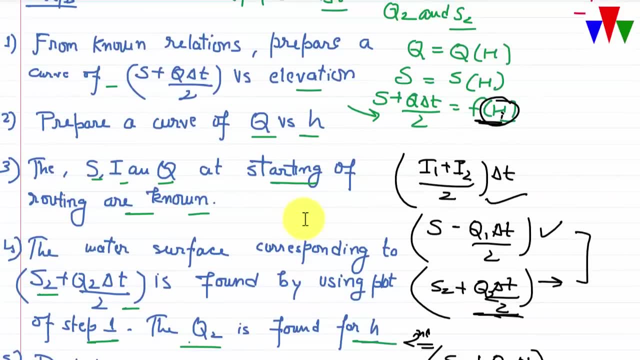 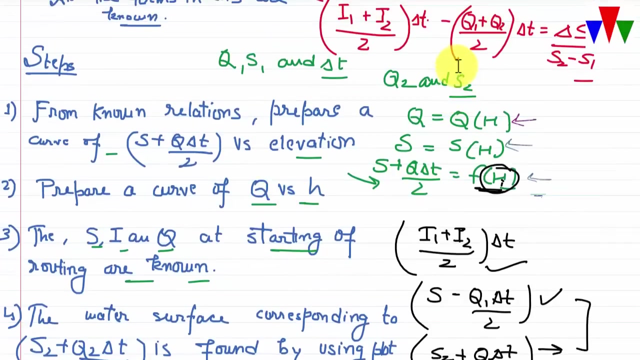 you once again the philosophy behind this modified pulse method routing in this equation. you have to just focus here. you know, you know this thing. you know: discharge as a function of H, today's function of H and this function as a function of H. what you have done, you have, you have calculated this thing. 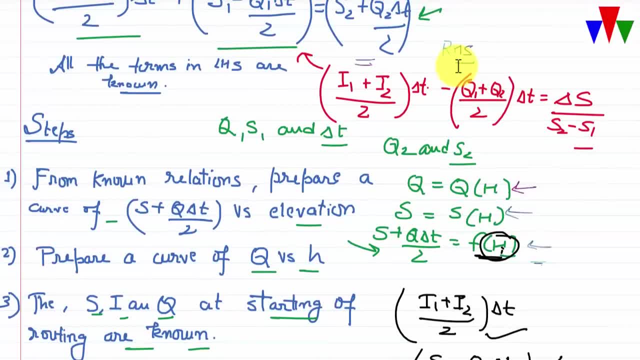 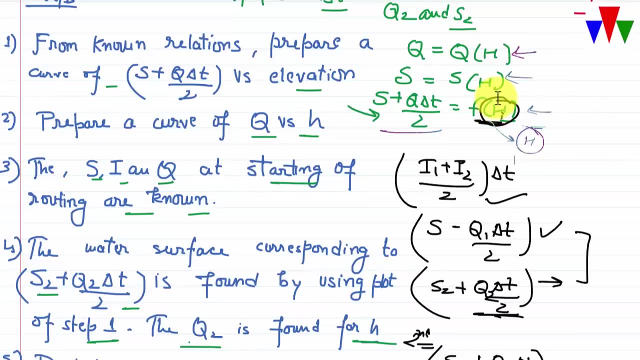 from. you have calculated this RHS by having the values of LHS. so you know RHS, this whole value. now this whole value put in here. then find H, what is H? so you know the H is found. at the same time from H, outlet discharge is found using. so, if you 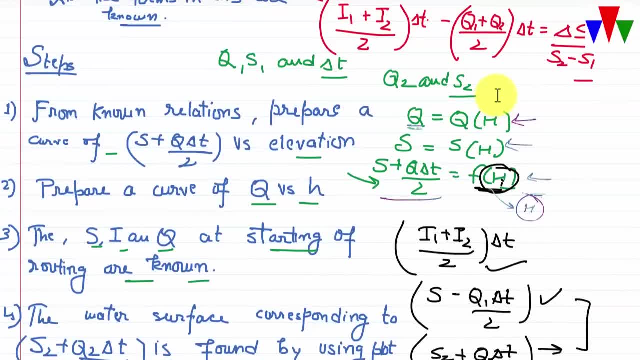 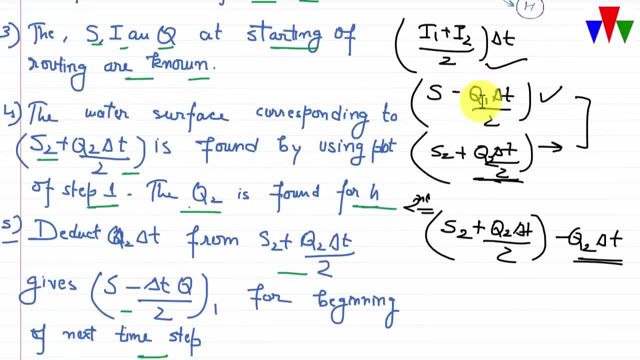 know each, then you also know Q. what is that discharged at that time? because that is the function of edge, so that discharge will become our. you know it is Q 2, so you know Q 2. you know delta T, so you, you, basically, you know everything in. 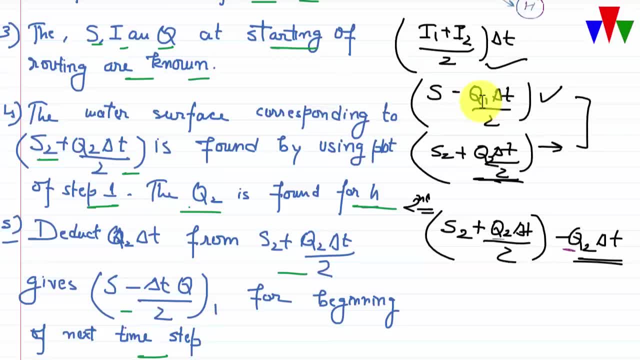 this and then you you subtract this from this to get the second equation. basically, these types of questions can be done using tabular method, which you can find in any good book. so the concept behind this is very simple and it will take some tactics for you to get through. 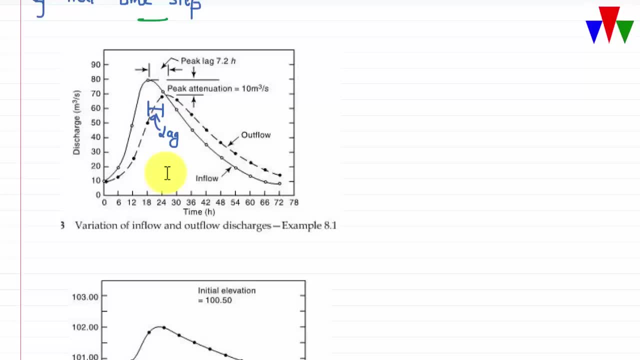 it now. let us see one example that what the routing does to our inflow hydrograph. as we see that this is our original inflow. you can see this, our inflow hydrograph, this rotor line. here we have peak of around 80 discharge meter cube per second and after routing we have attenuation of 10 cubic meter. 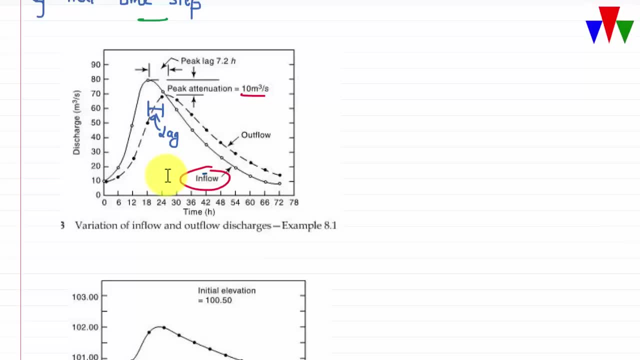 per second outflow hydrograph. and also there is lag. what does lag mean? lag means that the value of peak are separated by a time interval, delta t. there is some time between these two peak values. if these two value occurs just at one moment, then t will be equal. 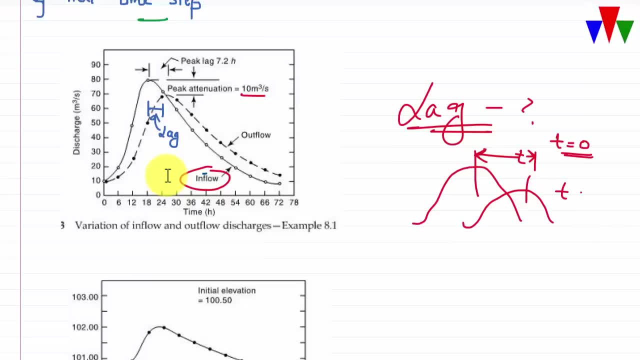 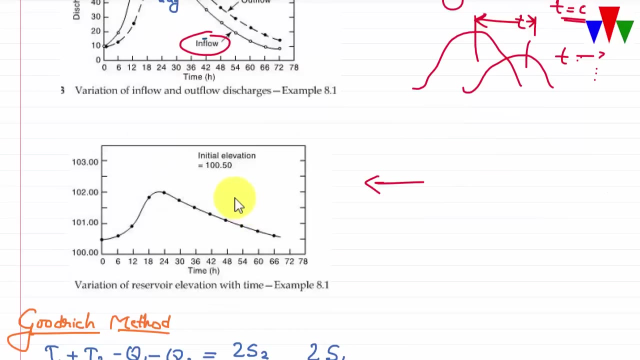 to 0, so lag will be equal to 0, but in our case t has some value and in this case it is 7.2 hours. it means the maximum peak for outflow takes place at 7.2 hours after the inflow peak, and this is example of variation of reservoir. 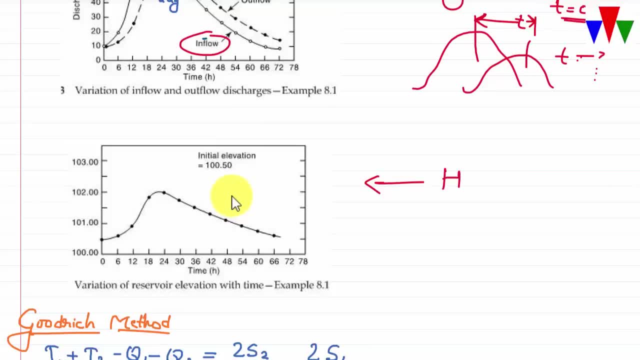 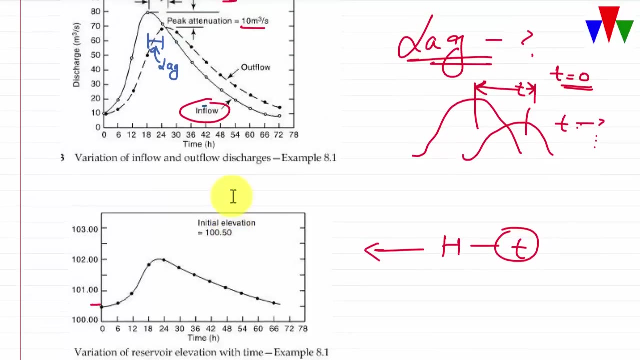 elevation with respect to time, that is H as a function of t, that how the reservoir elevation varies with respect time. you can see that initially values here, but suddenly, suddenly, at this point where the you can see inflow peak is here, the reservoir is at its maximum level. one more method of channel routing. 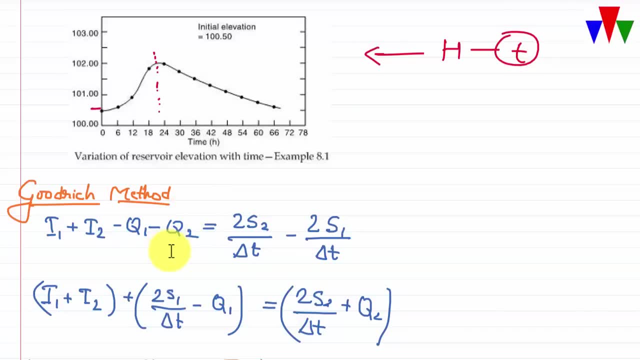 storage routing is goitris method. third, it is just another way of rearranging the earlier equation that we have seen in all terms in LHS are known and that on RHS are not forgiven time increment at 30. so you have to determine RHS side after time T from LHS side in. 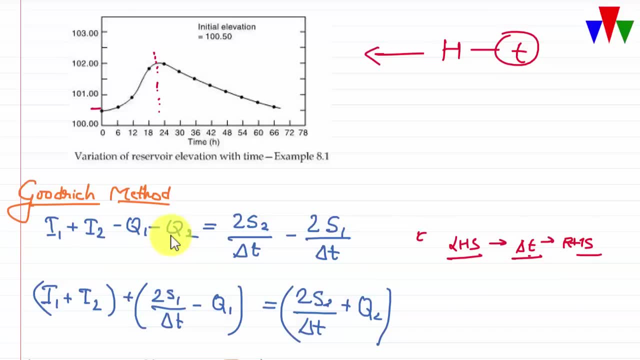 this: 2 s by 2 s, 2 by Delta T plus Q 2 is determined from storage elevation discharge, which is a function of elevation. similarly, for calculating next time increment, initial value will be this: 2 s by Delta T plus Q 2 at time 2. 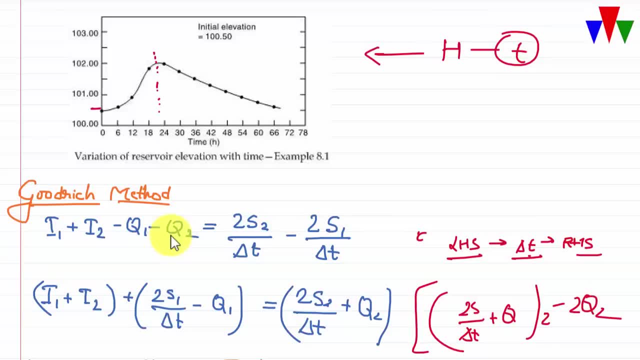 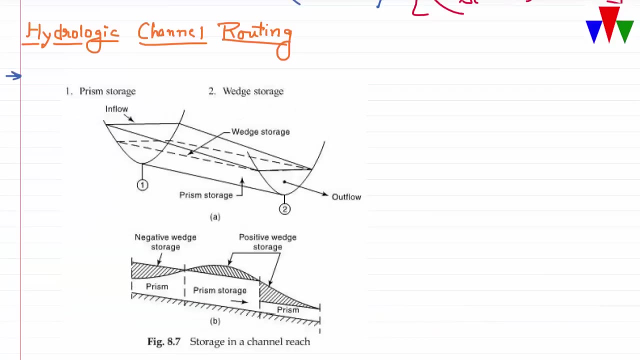 minus 2. this thing will be your step for next increment. so the concept is basically same and we have to just another way of rearranging continuity equation. after studying storage routing, let us see about channel routing. so by now you know the difference between storage routing and channel routing. in storage routing, you know we store a. 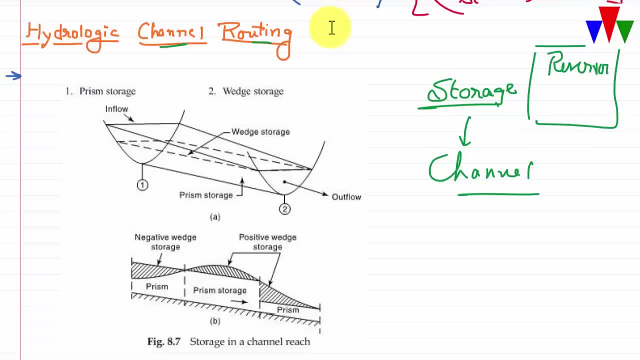 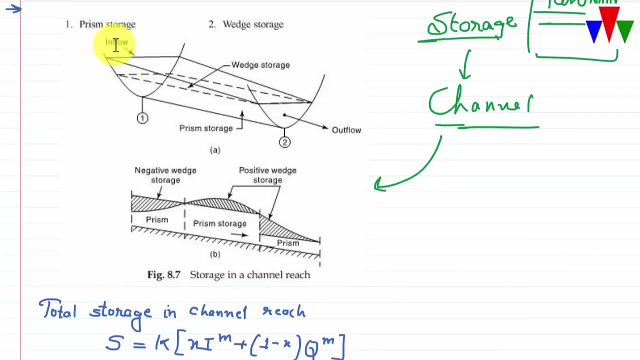 water used in a reservoir or any structure behind which water level can rise. but in channel routing we allow the water to pass through a channel and by allowing to pass through channel we get this type of routing method. in this you can see that we we assume that flood wave will. 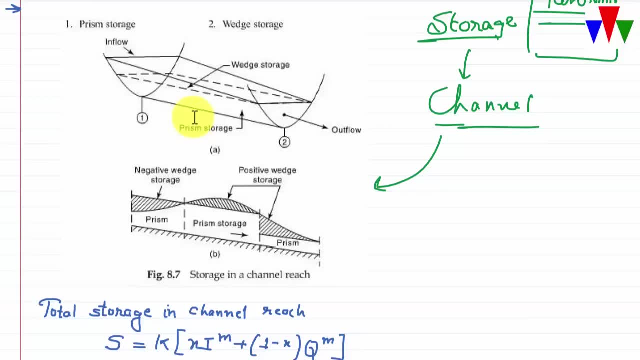 be reduced in magnitude and lengthened in time travel. that is annulated. the storage and between two sections. so this is basically, this is just your river or channel, you can say, and this is your section 1, section 2 and the storage in channel reach is divided in two part: prism storage and veg. 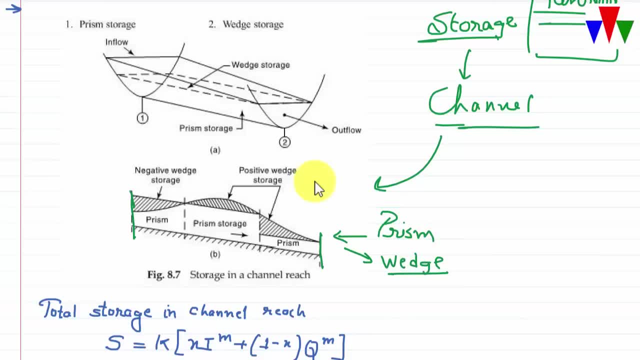 storage. so prism storage is that storage which basically, and the line is parallel to your downstream bed bed line, and veg storage, the volume above or below that line. this horizontal line is called as veg storage. so if this water surface is above your, above your line, then it is called as positive veg. 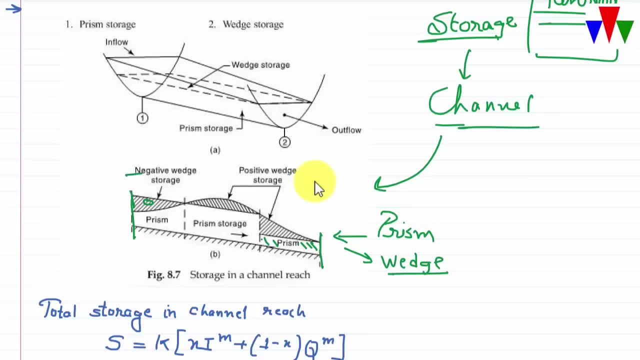 storage. otherwise in this case, like this, it is called as negative veg storage. so we have our prism storage here and our veg storage in this. these are just ways of defining your storage in your channel reach. during rising stages, the veg storage volume is considerable. it means that when the flow 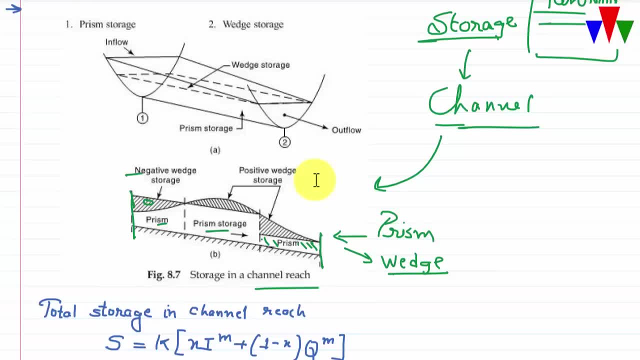 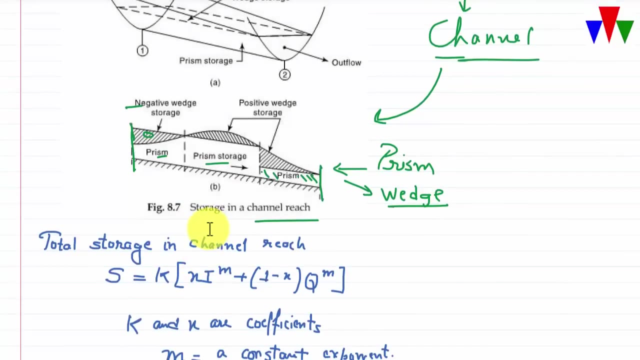 is rising, the water surface will not be parallel to your bed. as, in flow drops more rapidly than outflow, the veg storage becomes negative. in the case of stream flow routing, the solution of, basically, in this case, the solution is reservoir routing, because veg storage is involved and this veg storage is a 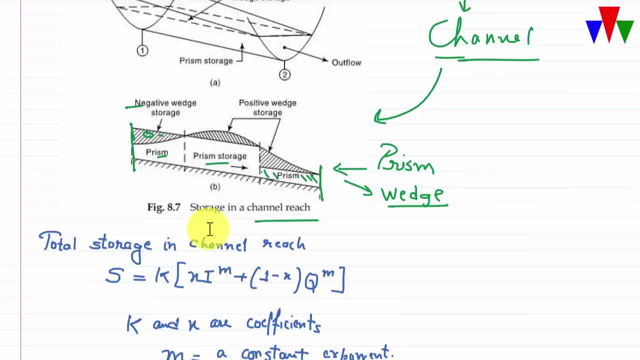 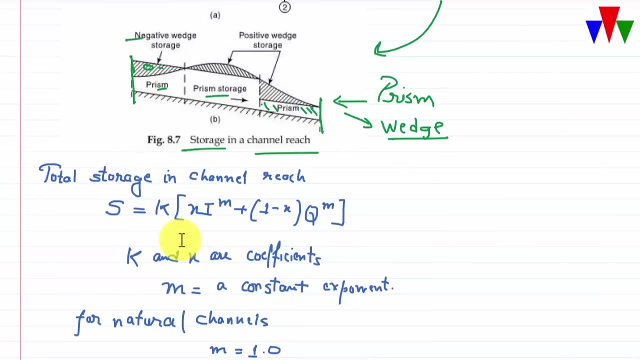 function of your input and output. so this storage of storage in channel reach plays an important role here. let us see one method which is known as muskingum method. here the storage is given by this function. this function is called as KQ. in this we- in this equation K and X- are coefficients. 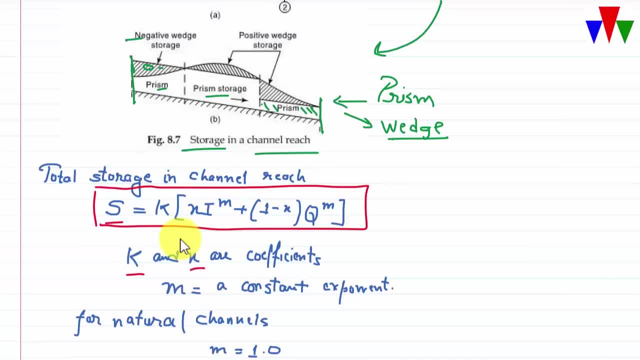 and basically X is known as a waiting factor. it takes value from 0 to point 5. the value of X depends on the shape of h. this: when X is equal to 0, obviously the storage is a function of discharge. only you know, X is KQ, M is a constant of which is used in exponent. M is 0.6 for artificial. 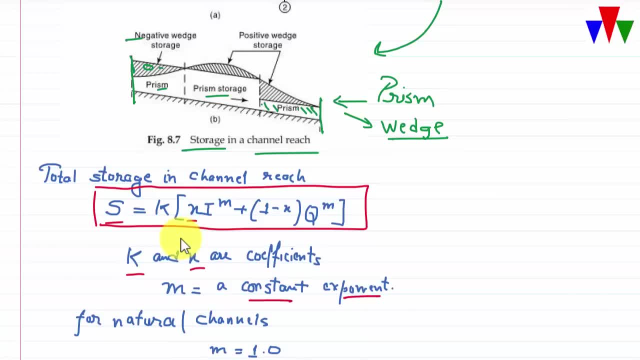 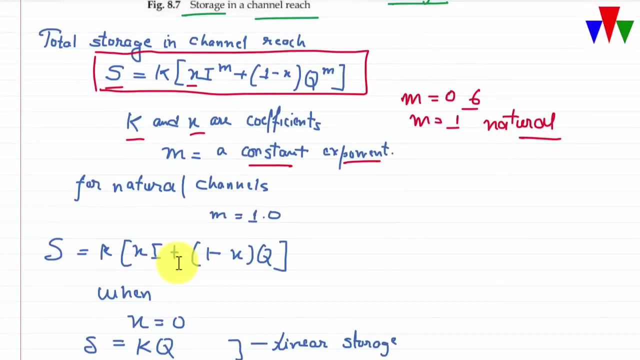 KQ. M is a constant of which is used in exponent. M is 0.6 for artificial shell rectangular channel or m is one for natural. such a storage is known as linear storage. the storage is known as linear storage. storage varies linearly with the coefficient. k is known. 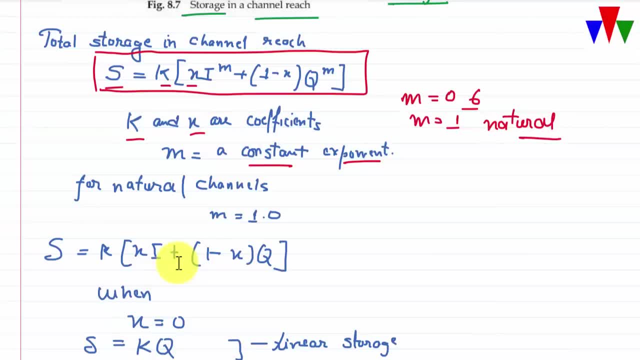 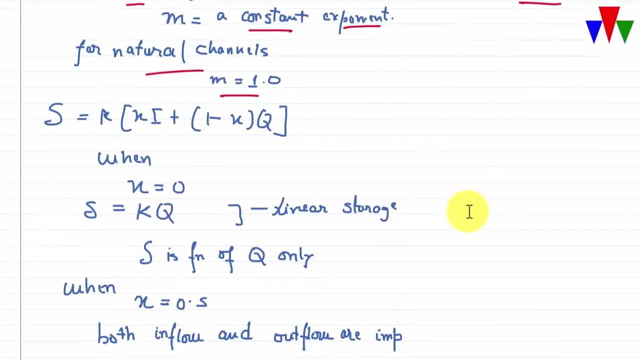 as storage time constant and has dimension of time. it is approximately equal to the time of travel of flood wave through channel reach and the value of k depends on length of reach, another roughness characteristics. so basically, this equation you have to remember and you have to remember all these constants and what are the values they can take. so let us see further the 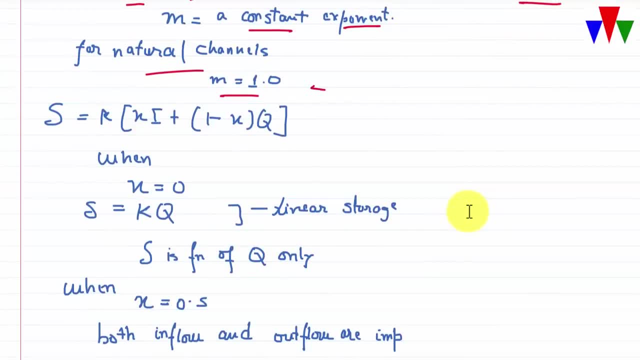 use of this equation. for natural channel, as we have seen, m is equal to 1. therefore, this equation become: s is k, x, i plus 1 minus x times q. for natural channels, when x is equal to 0, that is, when weighting factor is 0, then s is a function of. 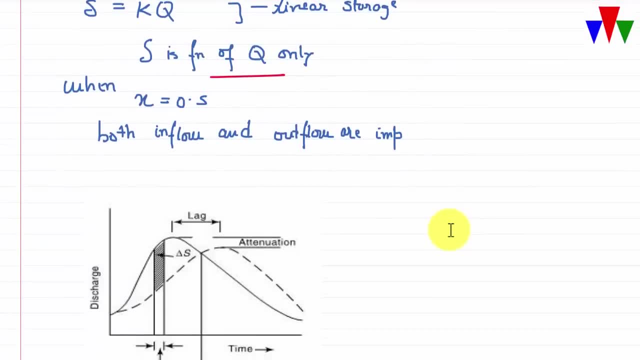 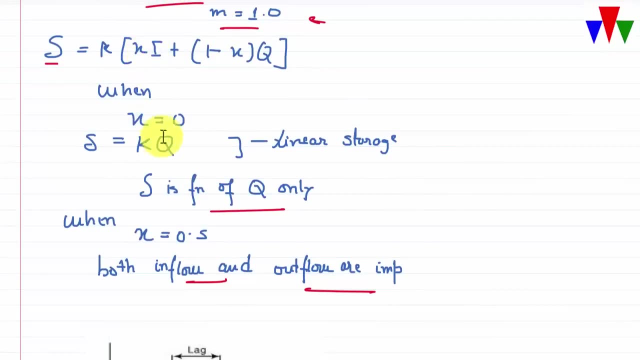 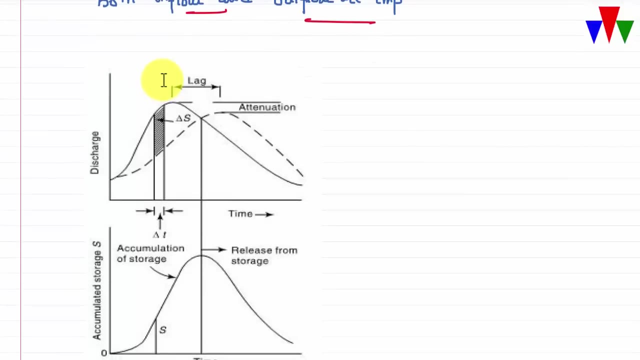 q only when x is 0.5. both inflow and outflow are important. it is the weighting factor of with respect to inflow. if x is 0 means inflow has no role. it is the storage, is the function of discharge only. so you know x and 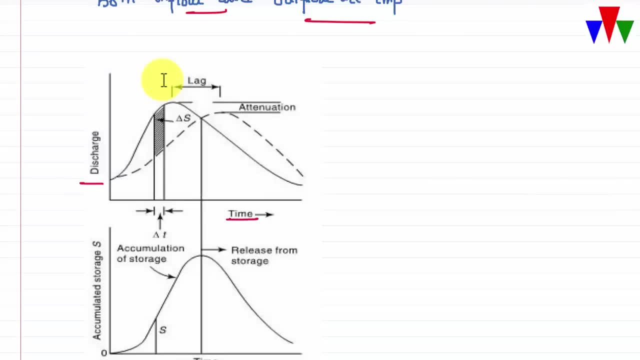 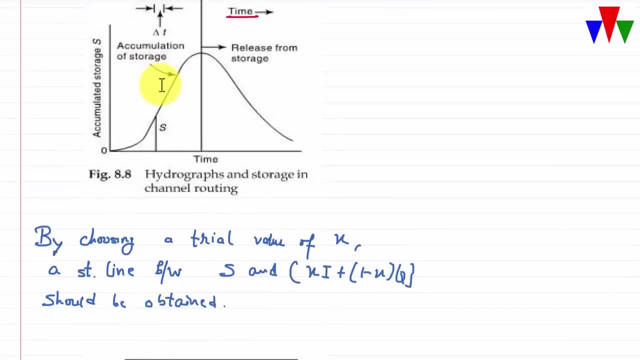 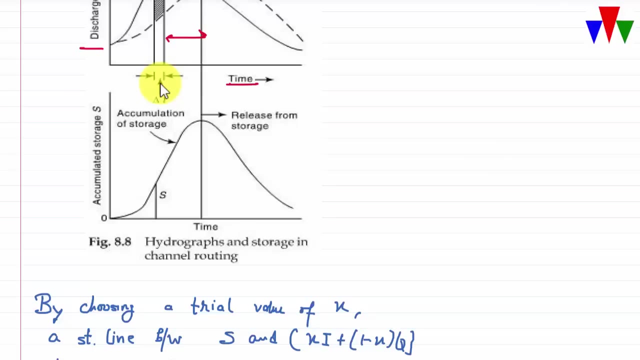 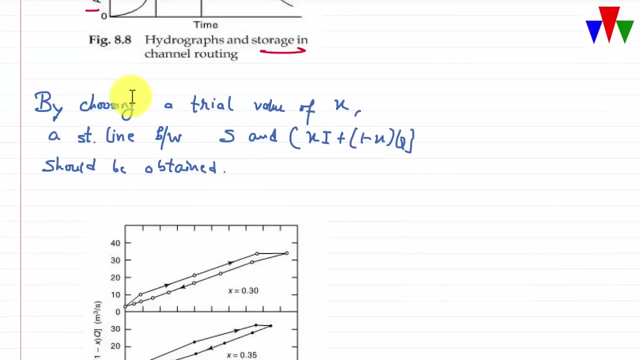 with respect to time, here you have attenuation, that is, the peak is, the peak is reduced, and also, with respect to time, there is lag and we have accumulation of storage. with respect to time, then this is a simple graph which you will get in your channel routing. so how do we solve this type of equation and 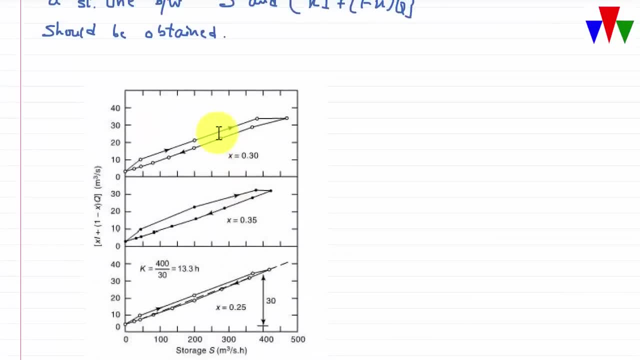 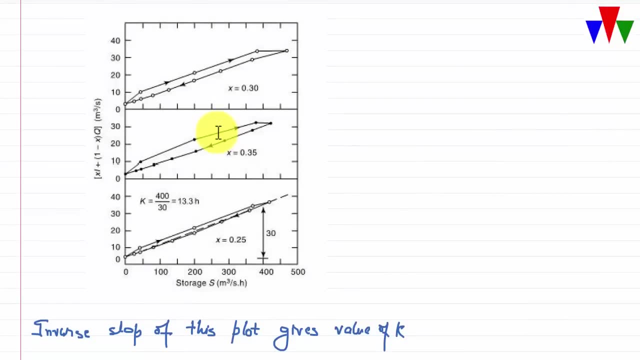 can be done, like we have said. seen in reservoir ID, you can see that we have plotted by selecting X plus 1 minus X cube. this function we have plotted with respect to storage. I have we have value of K here, X here for different X values. we have plotted storage function so inverse of the slope of the plot value. 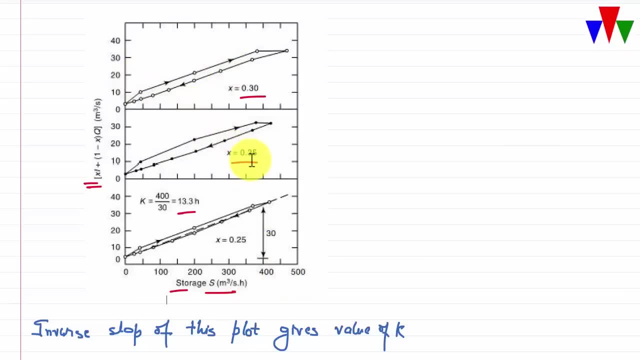 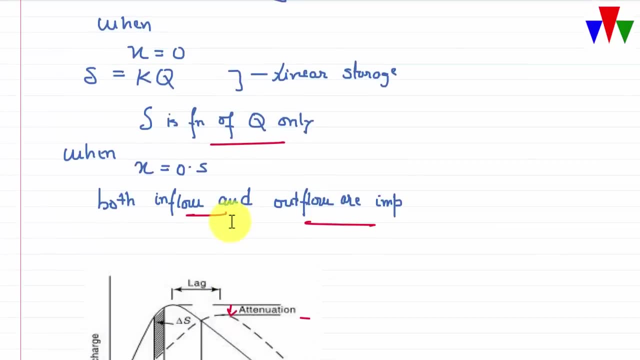 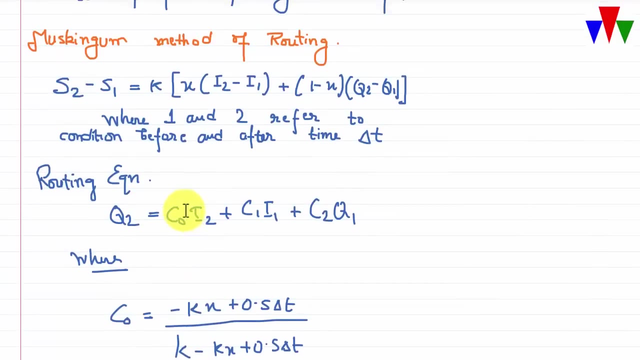 gives. so if you have plotted this, the inverse of this will give you a value of K. now let us see the Muskingum method of routing. this is Muskingum equation that we have seen here, and now we will see the method of routing, Muskingum method. 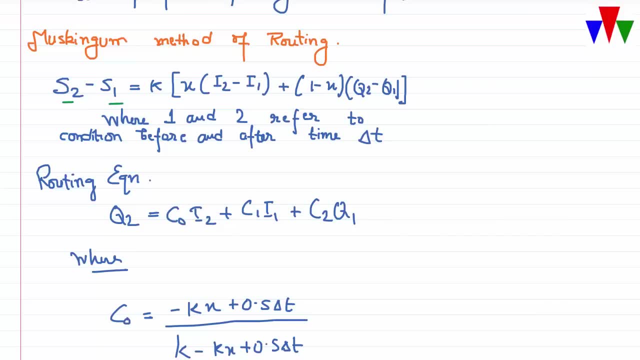 of routing says that your s2 minus s1 is K times I. 2 minus item plus 1 minus X, Q 2 minus Q 1. in this we have taken natural channel because our value of M is equal to 1 in this equation. okay, and 1 and 2 refer to. 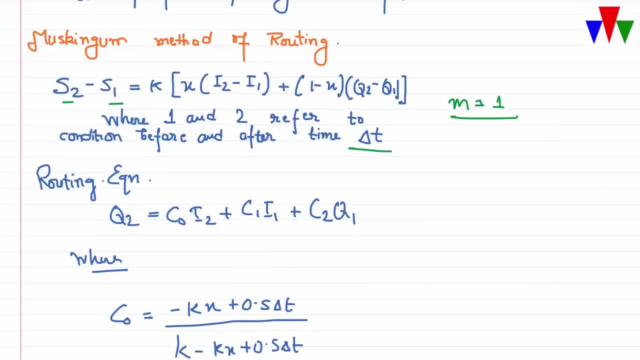 different conditions and for after time. delta T routing equation is from these two thing we can. we can say that Q 2 is finally function of C, oh, I 2 plus C 1, I 1 plus we 2, Q 1. in deriving this equation, one more equation has been used along with this. let us call it as a and. 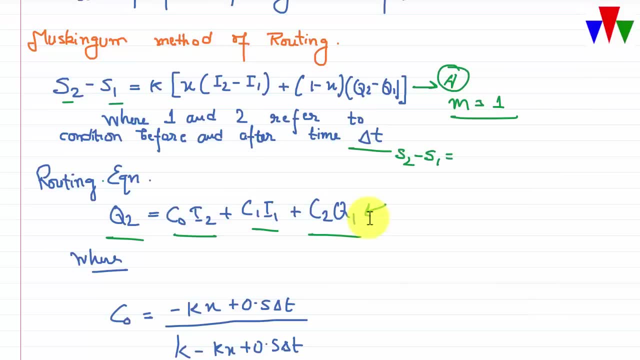 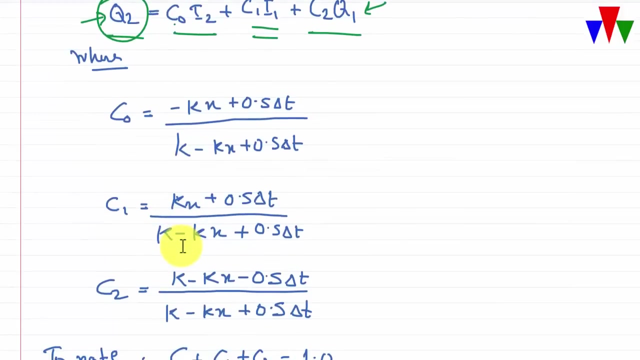 as we have seen, at least a test, 2 minus s 1 is i 2. i average delta t minus Q 30. so these two things, these two things, we get this equation routing question that we will get the value of discharge time interval 2. so this is C naught, C 1, C 2, we have to. 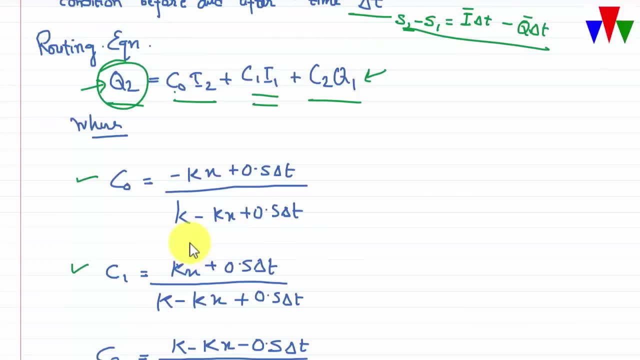 remember the value of these coefficients, because there is no other way. C naught minus K, X plus 0.5 delta T, and likewise C naught C 1, C, 2. you, when the value of K and X are given, you will be able to calculate these two and then substituting. 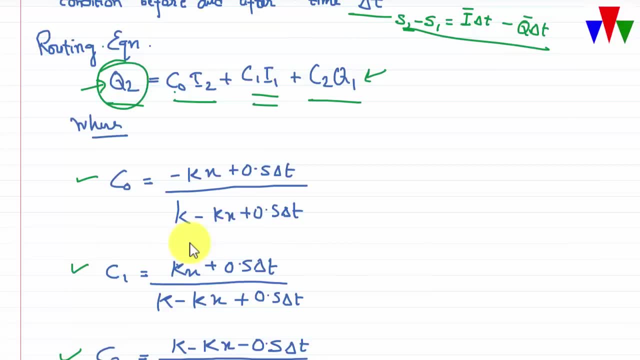 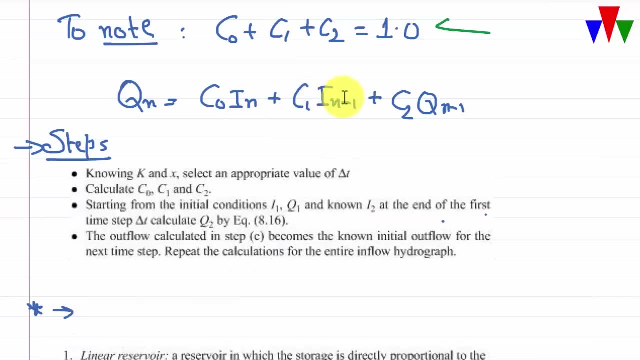 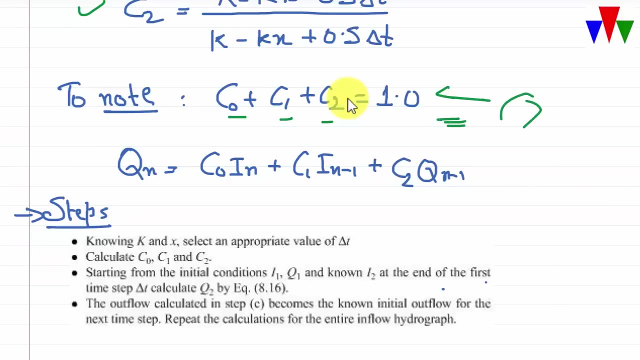 the value of these two, you will be able to calculate Q 2 given your value of Q 1 and I 1. so one thing to note is that the value of C naught plus one thing to note, that the value of C naught plus C 1 plus C 2 is 1 in this equation. so for nth time, 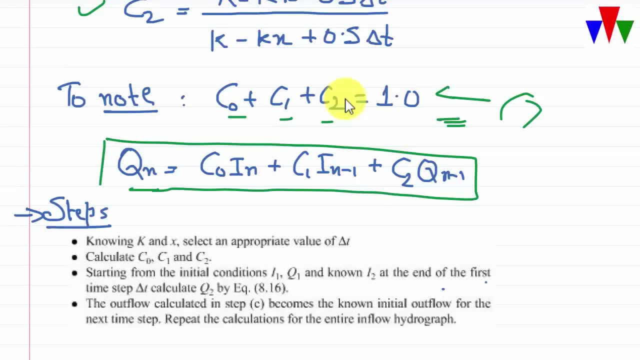 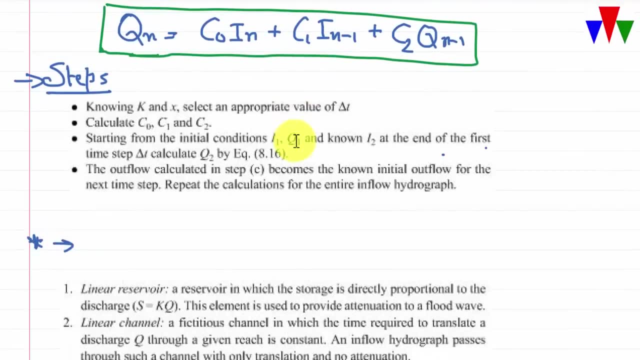 interval we can define the charges function of like this. so what are the steps to find this routing method to masking equation? we have to select the value of Delta T because we know K and X. okay, so we select in 30 time interval, through time interval, delta TV. we calculate C naught, C 1 and C 2 because, as seen in this, 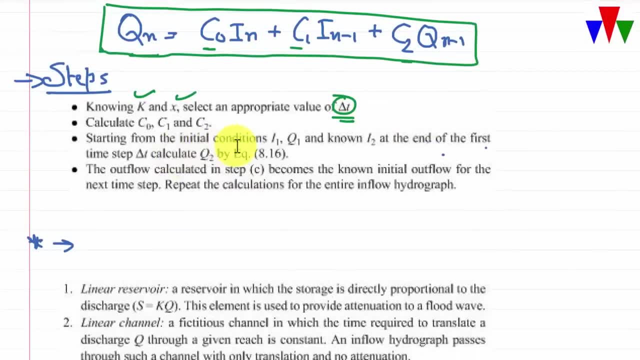 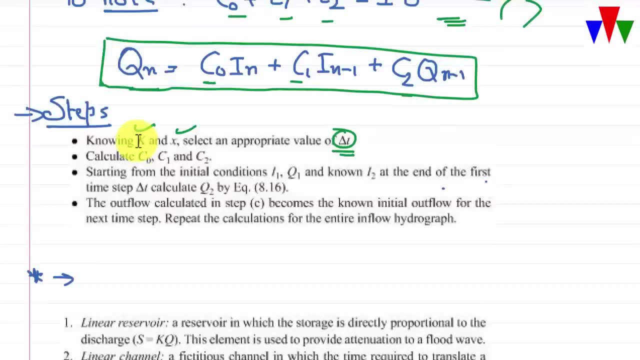 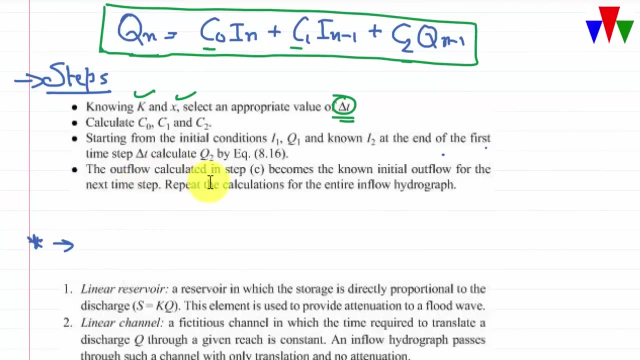 equation. you can calculate this and starting from initial condition of I 1, Q 1 and known T 2, I 2, the end of first time step, calculate Q 2. it's very simple. we have to calculate Q 2, then Q 3, then Q 4, so the out outflow in becomes inflow. 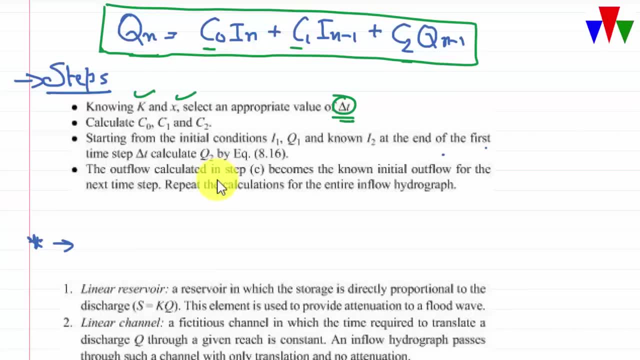 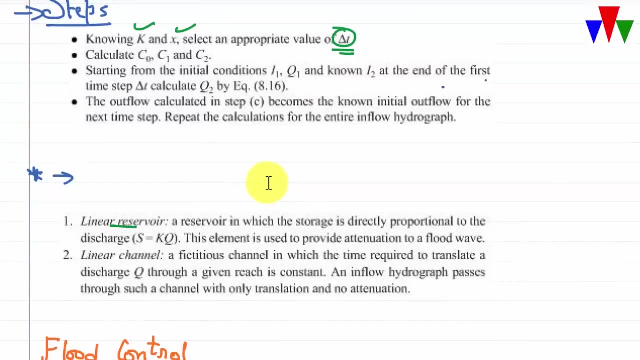 for the second, next time step, that it means that here your Q n minus 1 is input for your this outflow, Q n. so this is what it is saying. so we have to repeat the calculation for entire flood hydrograph. now we see that linear reservoir is a reservoir in which storage is directly. 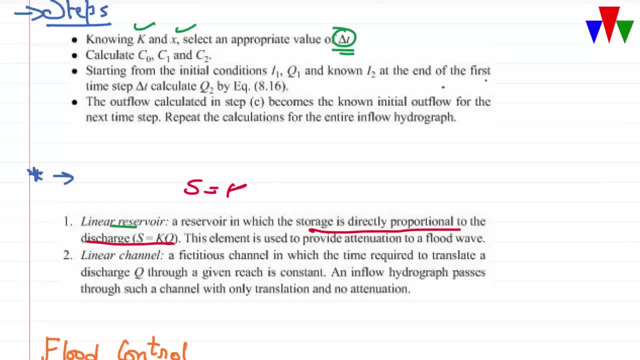 proportional to discharge, that is, S is function of Q only. this is called a linear reservoir. this is an important concept: linear channel and a fixed channel. it's not real in which the time required to translate a discharge Q through Q and reach is constant and inflow hydrograph passes through such a 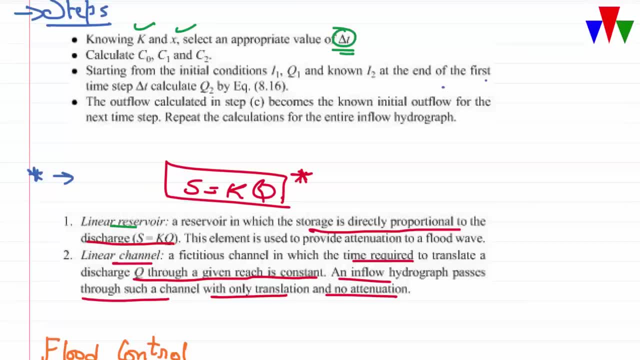 channel with only translation and no attenuation. but it says that there is no attenuation, that for in linear reservoir, this is your inflow peak, then this will be your outflow flow peak. in this, these two will be at same level. there is no difference in inflow and outflow and there is no. 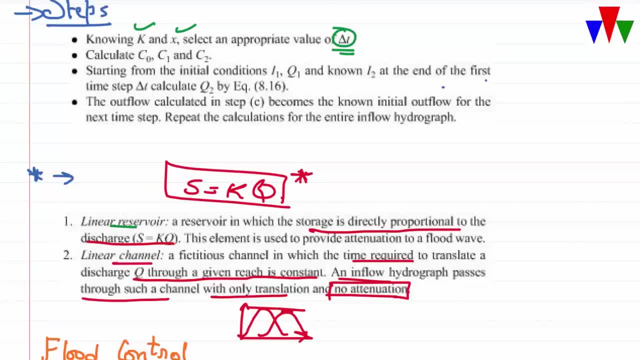 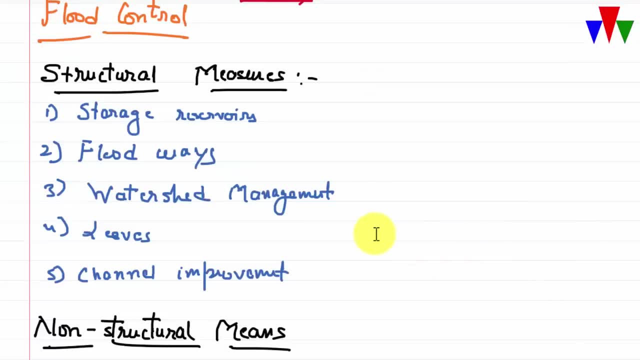 attenuation. this is called as such channels are called as linear channel. now let us study some. now let us study some method of flood control. basically, flood control can be defined into methods, two-part, structural and non-structure means. so structural means, that is, we create some structure across the flow of river or channel. first is your storage reservoir. 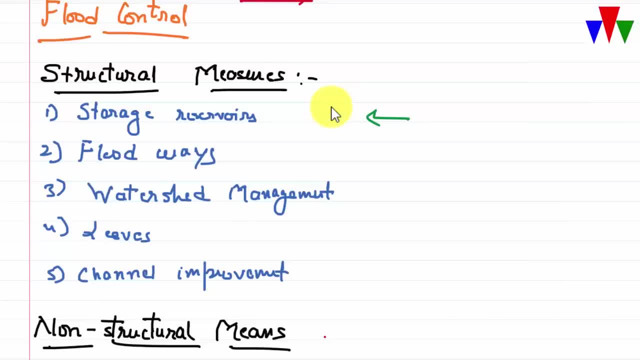 in this. these are very popular or very dependently used. and second is your floodways, watershed. what does this floodway means? floodways are natural or man made channels into which part of the flood will be diverted during high stages. so storage reservoir is clear, that is, we create a reservoir. there are a lot of. 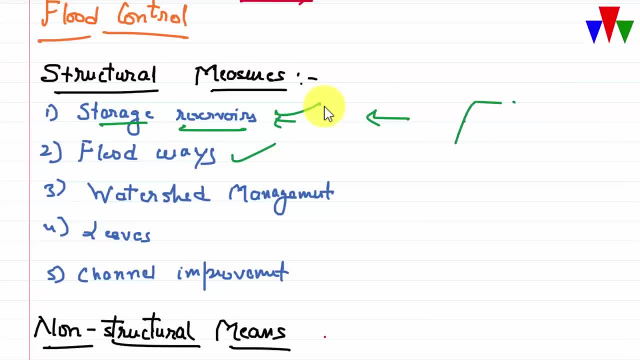 method for creating reservoir- most popular one is creating it and other hydraulic structures. then there is flood base. now you have watershed management in these. watershed management is basically involves a lot of work in your watershed area, such as widening or deepening of channel, reduction of channel roughness. the other methods, such as vegetation, increasing vegetation. 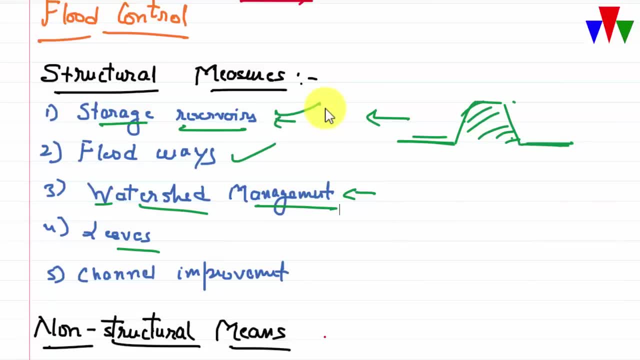 making check dams so you can use this method to increase percolation or basically delay runoff, reduce erosion, plant trees of forestation- these comes in water management and leaves dykes or flooding embankment. basically, this is your river. then these these two and say that a high 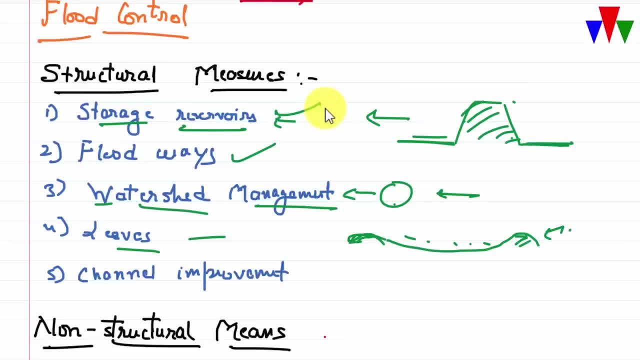 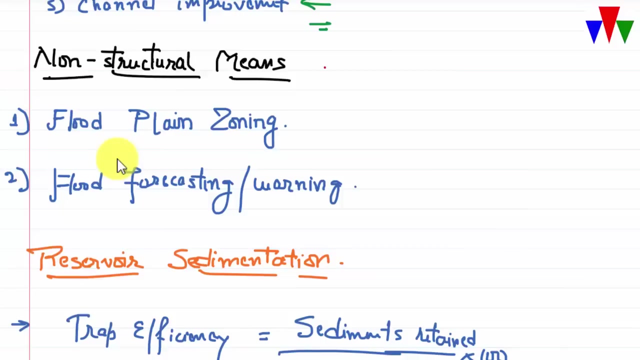 bank on the sides of the river. this is called as, and there are methods of doing channel improvement where you can do increase cross sectional area of river, you can clear vegetation, you can increase slope like this. these are structural methods for flood control. non-structural method include flood plain zoning. that is then 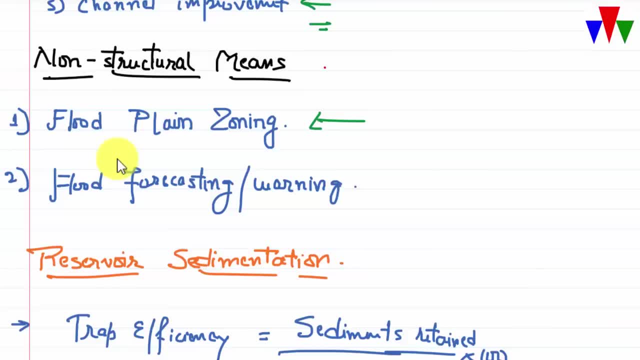 using flood prone area is regulated. this means, if your river is this okay, and we know that maximum extent of flood plain is here to here, the river can flood, so we will not allow settlement in this area. you can make buildings here, but not here, and you can. 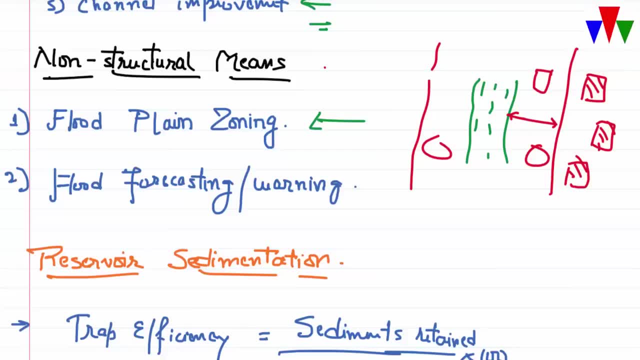 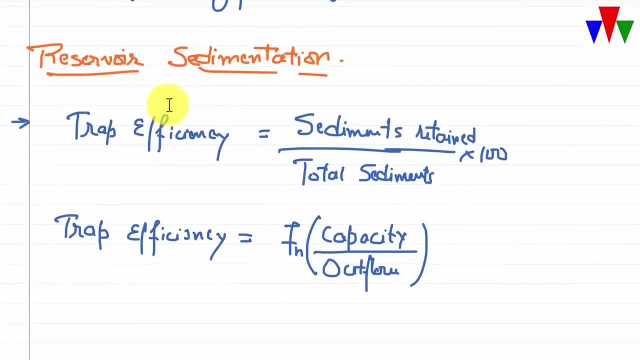 regulate the use of these flood plains so that in future, if flood comes and human life and the resources are not disturbed. now let us look at one more concept of reservoir sedimentation. the deposition of sediments in reservoir is called reservoir sedimentation. what does this mean? that if you have this time, 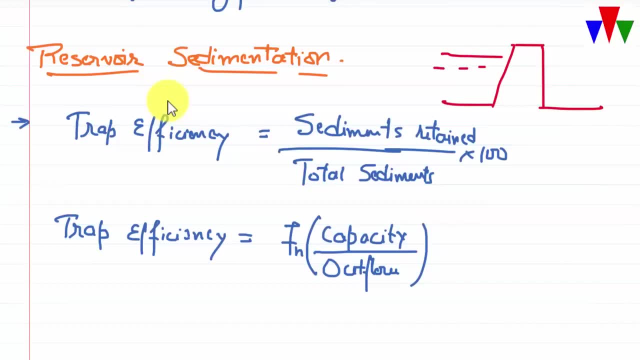 and you have at that time. that is means it is a solution at what happens to give aluminium but water will have gone. Warning when the water is not passported. all basically water and the physicians mentioning from otherперiod was also. it is part of the situation. we come to the origin of Marine. 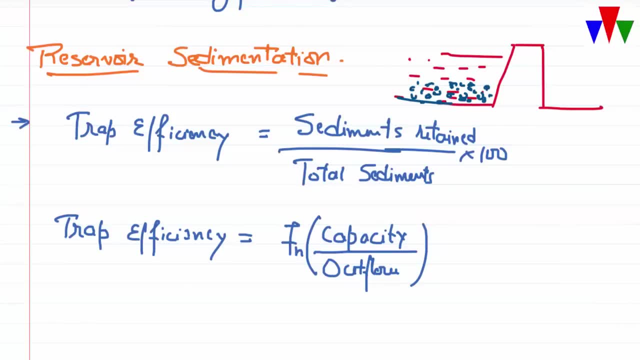 penguins in india. we imagine Japan straightaway. absolutely we and water carrying a heavy and also about 40 reduce from the shape of لكنware is about to change down. there is no problem to take place behind this, behind this attitude will take place. as in the water has stopped here completely, so the, since the water is not in motion, the position of reservoir sediment will be taken place. and since river has stopped here completely, so the wes release the water. 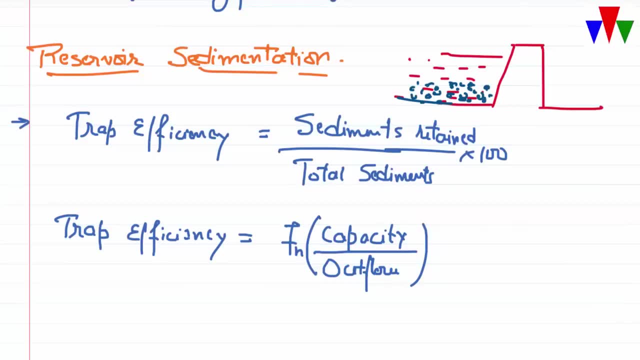 it reduces the available capacity of reservoir useful life of as more and more sediments occur, average velocity capacity of reservoir decreases storage capacity. so with continued sedimentation a time will come when the reservoir will not be able to serve its purpose that so much of silt will be deposited then that 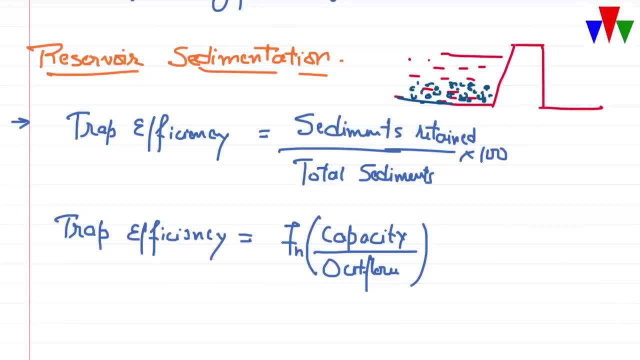 the purpose of creating reservoir itself will be defeated. so the rate of sedimentation depends on trap efficiency. this is a concept where we say that sediments retain with respect to total sediments. it's called a stress of their efficiency. so the lower the traps efficiency, the better it. 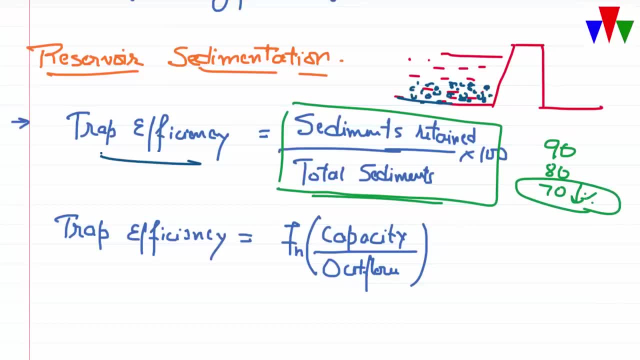 is so. if we have 70% traps efficiency mean 30% of the elements are going out. based on the observations, it has been found that trap efficiency is function of capacity divided by outflow. with respect to capacity and inflow rate, you can say that trap efficiency then 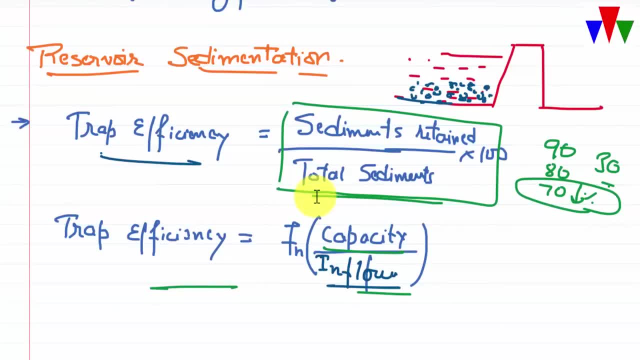 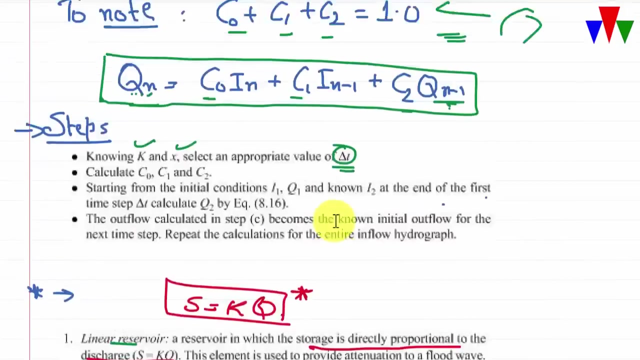 becomes the function of capacity with respect to inflow. this is a empirical exercise and it has been found that the function is like this. so now we come to the end of this chapter and I have very briefly explained you this concept about flood routing. so flood routing, in this we have seen our concept with respect to hydrologic routing. then 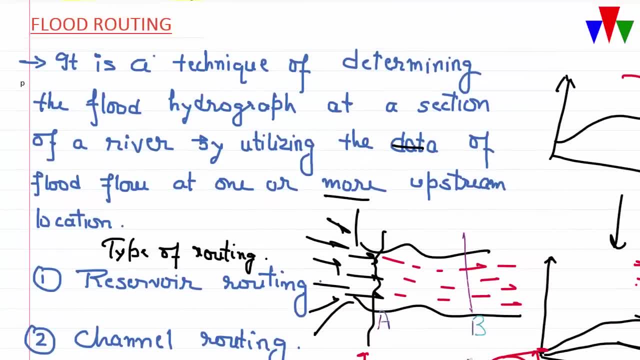 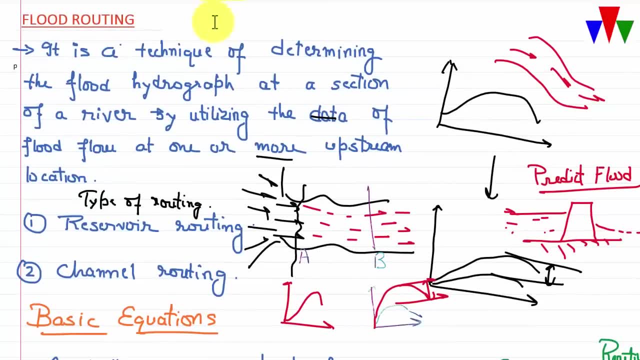 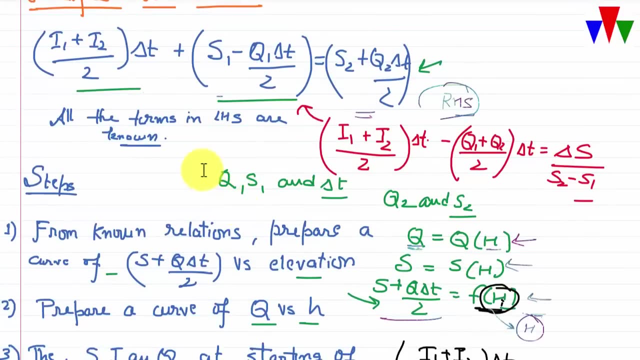 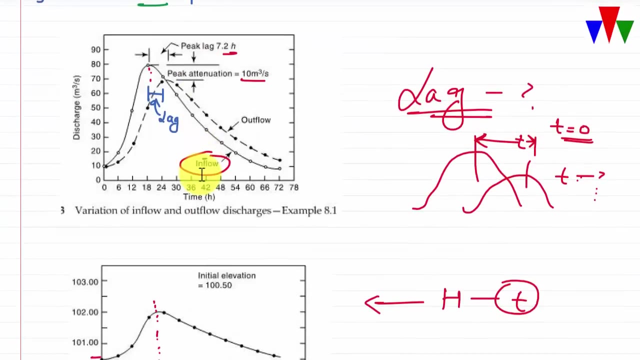 channel routing, then how the all the things fit together, and various phase in which we can calculate output, flood, hydrograph and how much peak will be attenuated, and what are the various methods of storage, routing and channel routing. so these concepts are not very difficult and I expect you to go through some 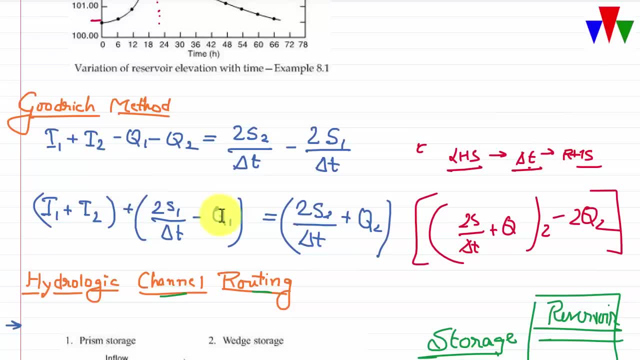 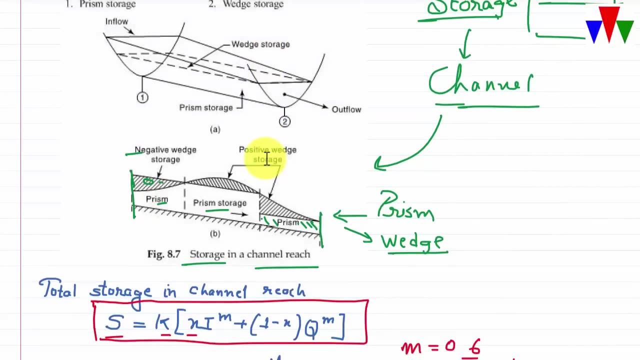 examples in the book, because these all examples will be based on a table like format and just by step by step, you will have, you will be calculating these values and then, with respect to that, you will get your discharge values, whatever. whatever function we want in hydrologic channel routing. 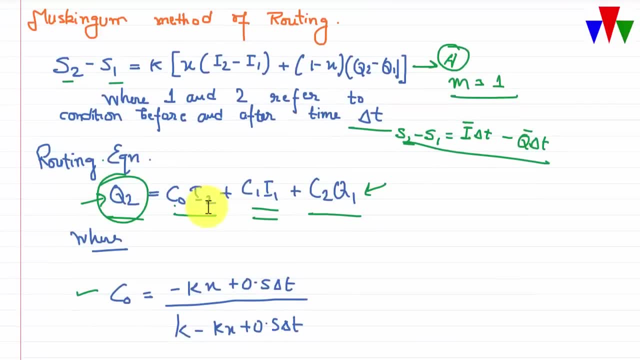 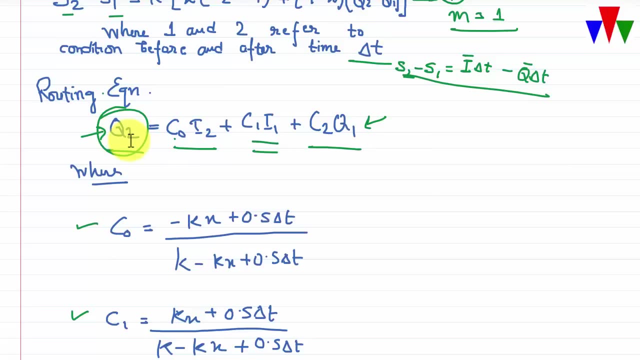 we have seen masking equation, and there I have also to learn these three coefficient values, and then the routing equation will be function of these three and the qt value will become input value for the q3 time step. so these are very simple and easy things to understand and more.